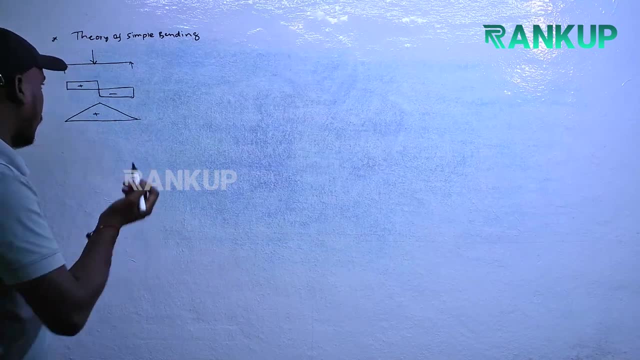 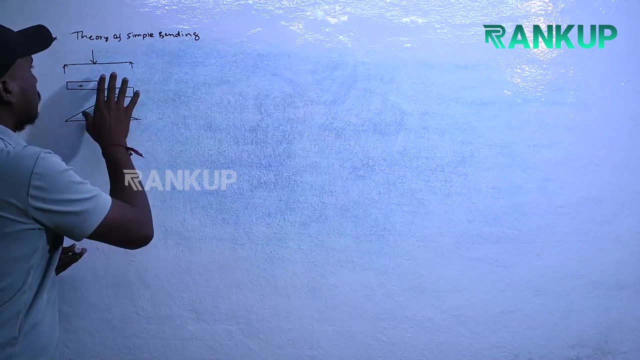 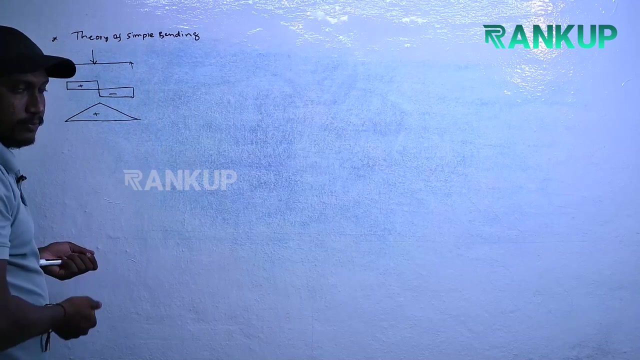 So what happens internally to the beam is that the beam provides some resistance to the bending moment and the shear force. Okay, internal. Now, when the load is applied, it bends. So the beam has some ability to bend, It has an internal resistance. 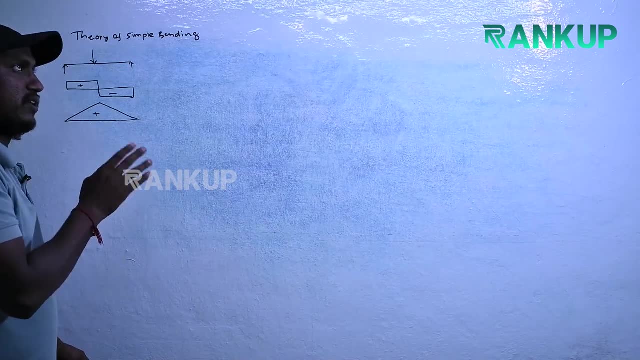 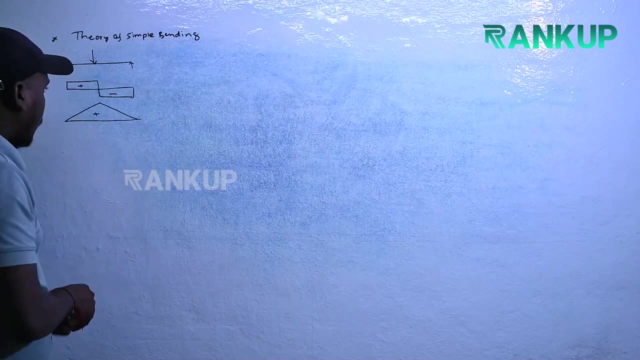 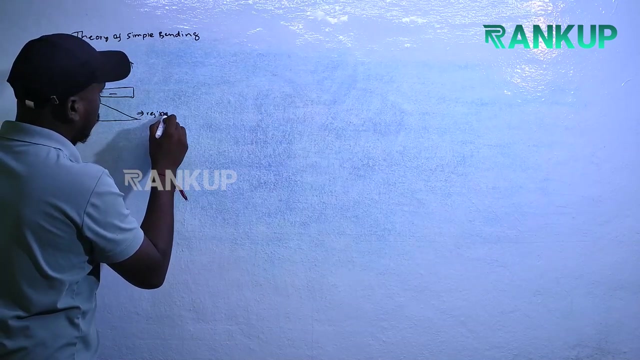 That resistance is opposite to the bending. It is opposite When it is opposite. what happens is that the resistance is opposite to the bending moment. When the amount of drop happens, the resistance is developed bending. We see the movement which is in the rounds is the bending. 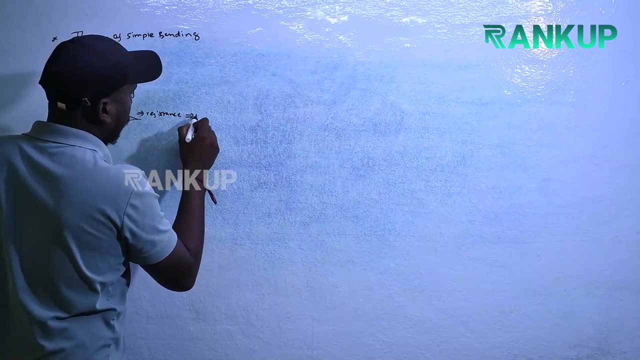 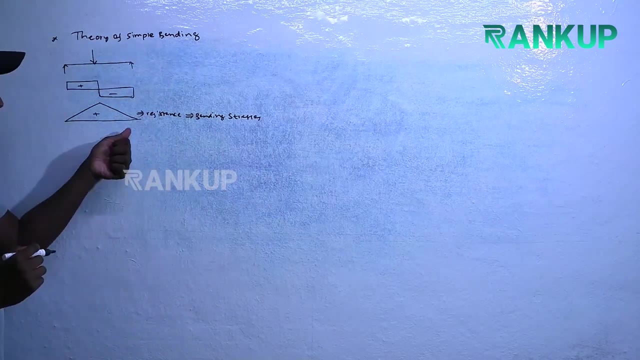 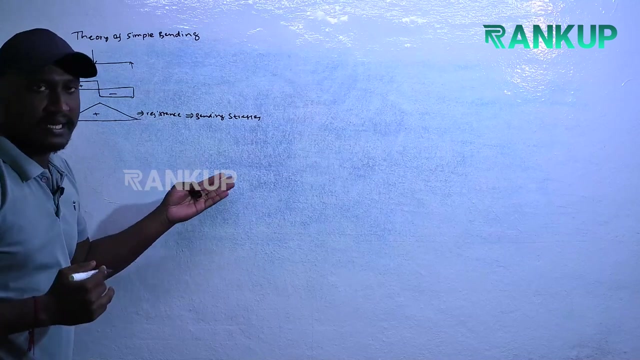 Can you imagine how the sensation is? Let's talk again. I am here because we are going to do strawberry fingurics. So this is bending. Okay now, Gerry. Developed against the bending. Resistance developed against the bending is known as bending stresses. Okay now. 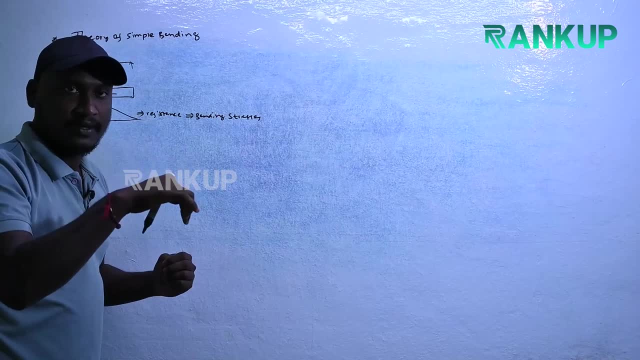 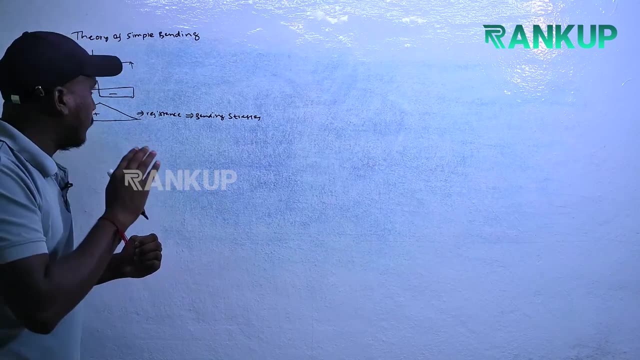 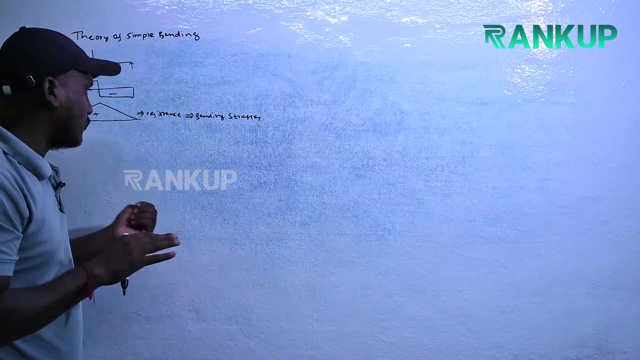 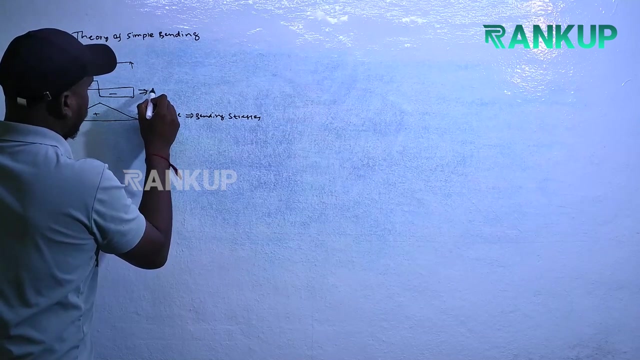 Whenever an external load acting on the beam, then the beam is trying to bend- okay now. but an Internal resistance developed by the beam against the bending- Okay now, the internal. that internal resistance is known as the bending stresses. Okay now, That's it Next. in the same way, in case the resistance developed against the shear force. 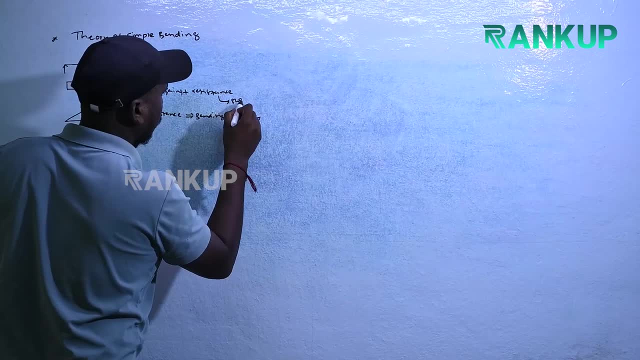 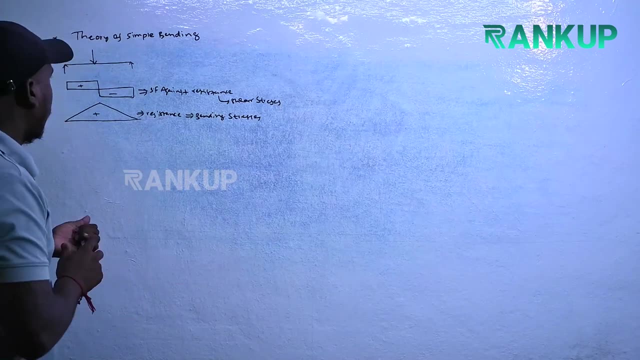 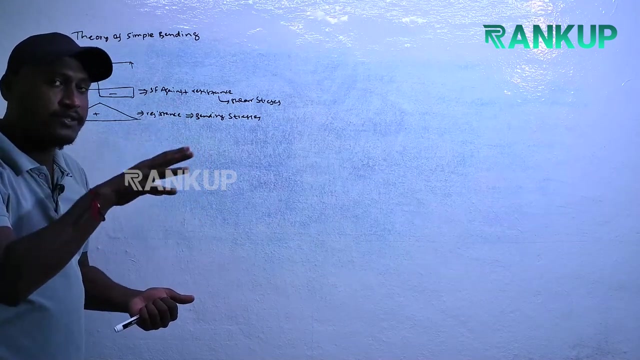 What do we call that resistance? We call it shear stresses. Okay, now we call that shear stresses. Okay, now Are you clear with it? Whenever external load acting on the beam, the shear forces are generated, the bending moment is generated. In opposite to that. 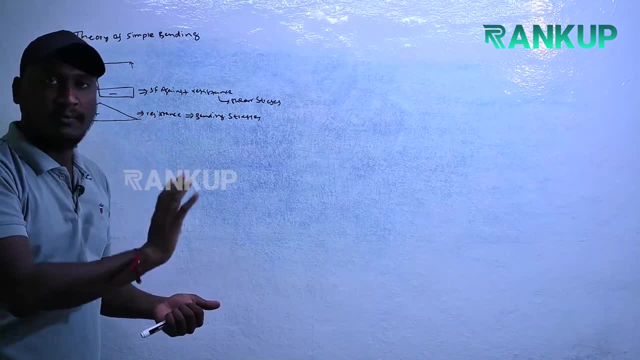 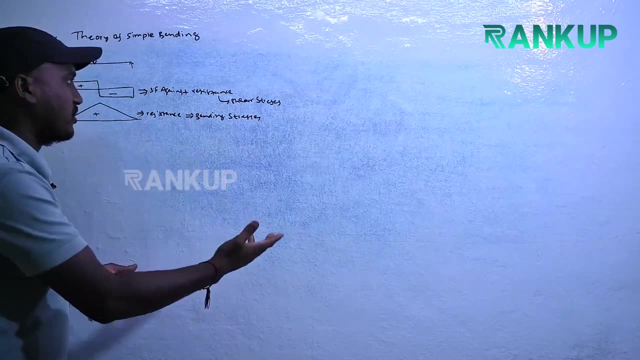 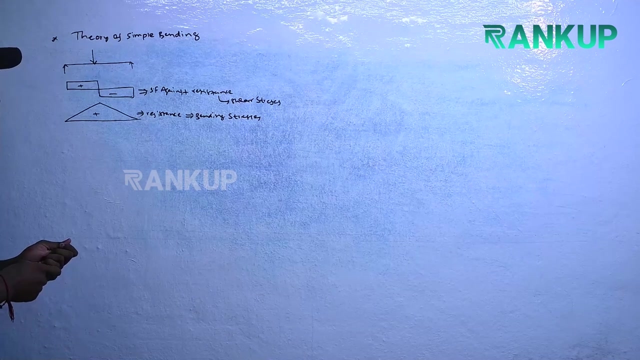 The resistance of the beam is Opposite to that. the resistance is developed as internal resistance. The resistance developed opposite to the bending stress is called bending stress. The resistance developed against the shear force is called shear stresses. Okay, now, Okay, next we have, next we have. 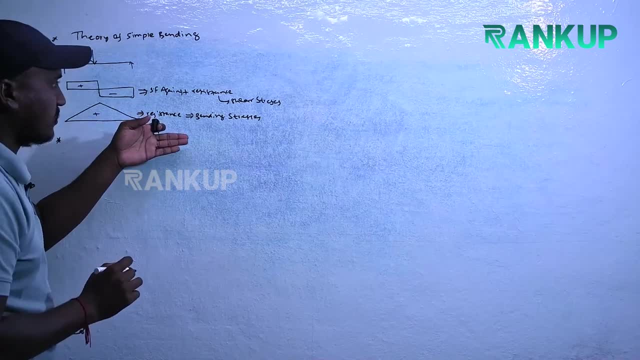 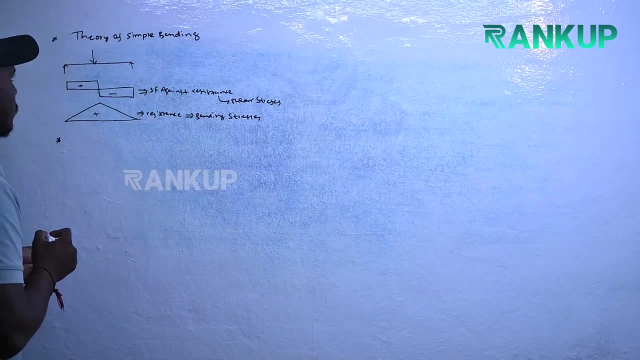 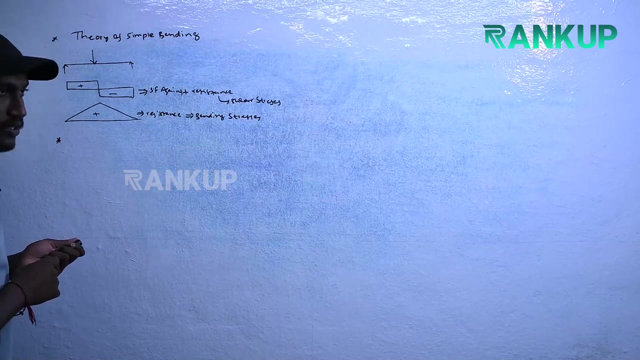 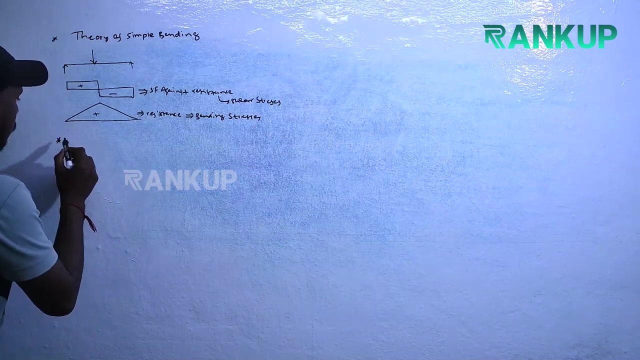 This is How the bending stresses develop against the shear stresses. That's it. Next we have Next, in theory of simple bending, Next we have. Next we have assumptions Next. next we have Before that assumptions, before that assumptions, we have some, we have some conventions. that is a 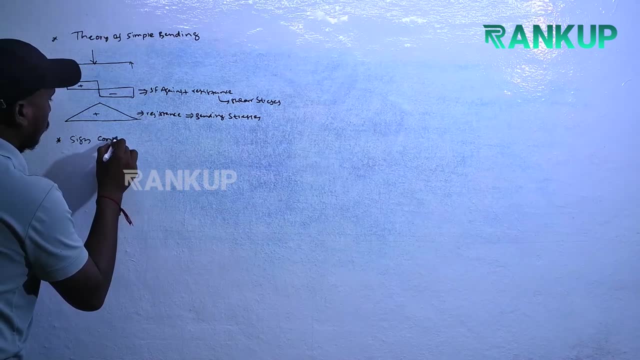 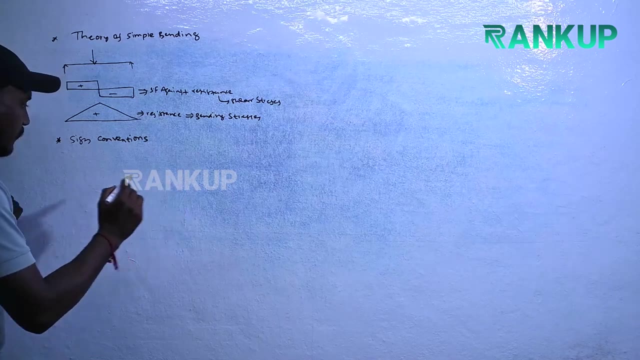 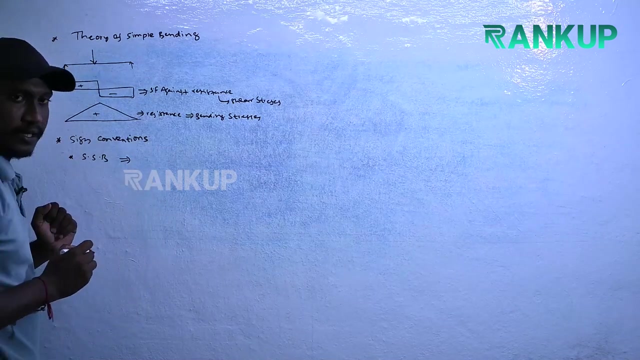 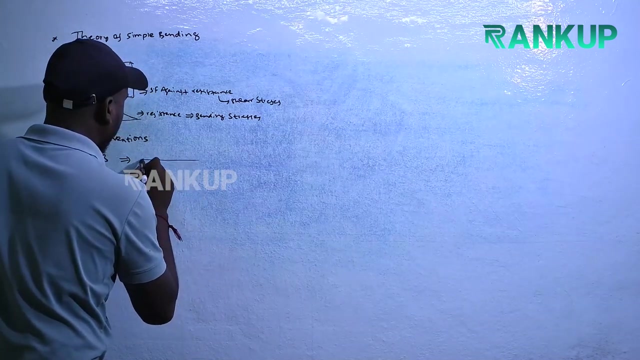 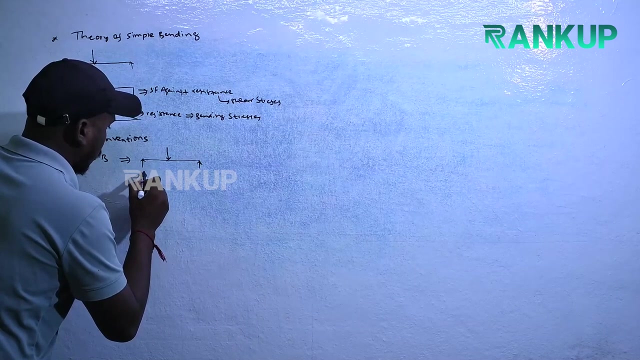 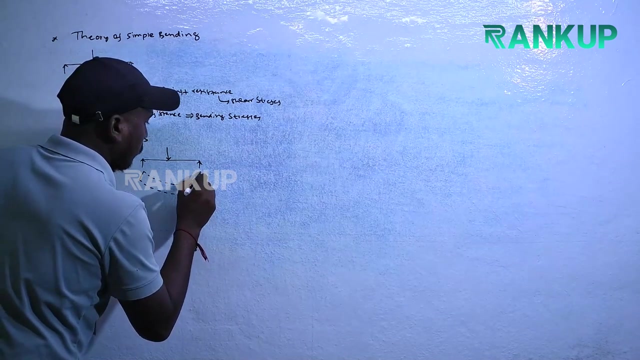 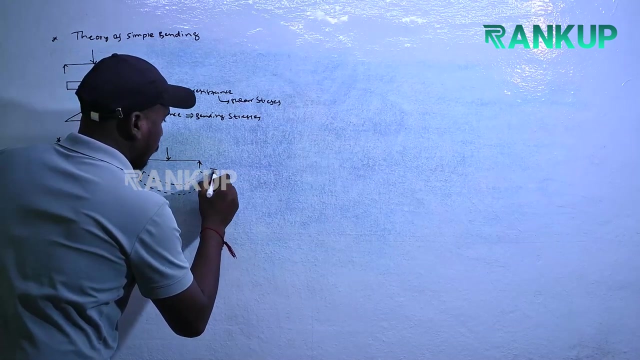 sign conventions. that is sign conventions. That is, sign conventions before Assumptions. we are going to sign conventions. Okay, In case 1, I am taking a simply supported beam. In this simply supported beam, the beam will bend like this. I have already told you that the bending moment is called sagging. 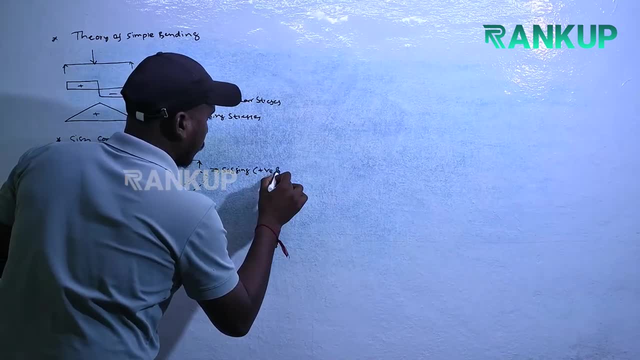 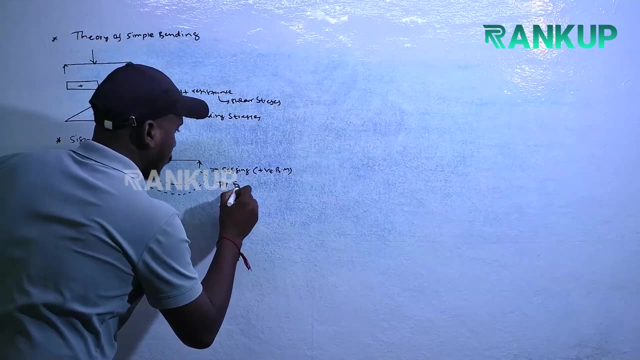 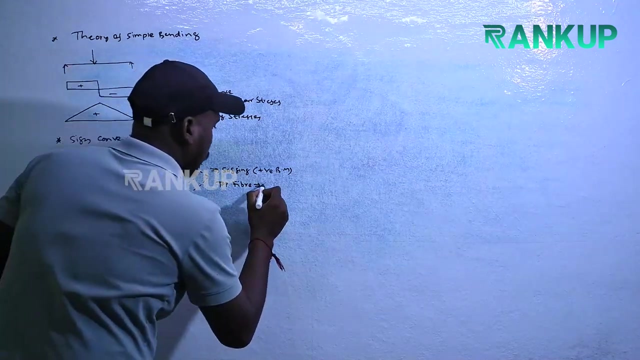 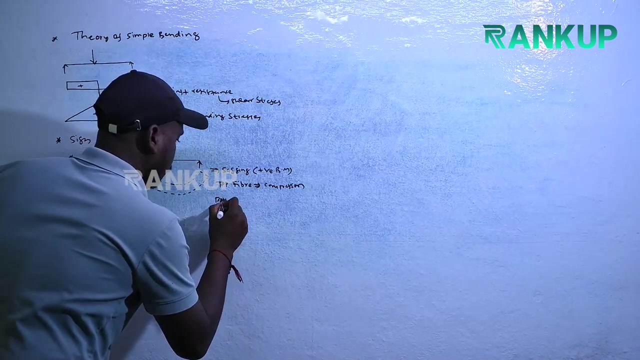 Sagging is a positive bending moment In this top fiber, top fiber. This is the top fiber. The top fiber compresses. So what happens to the top fiber, Compression happens? Next bottom fiber, Next bottom fiber. What happens to the bottom fiber? 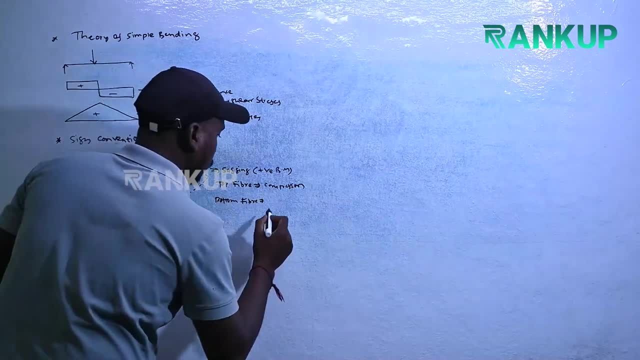 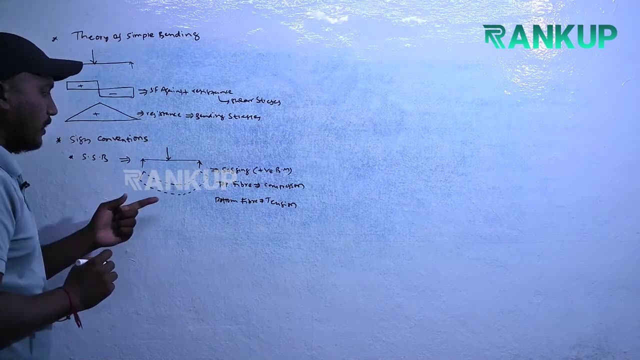 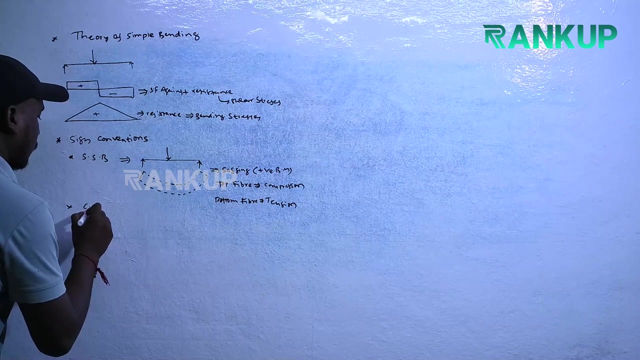 It tries to extend. So tension happens to the bottom fiber. What happens to the bottom fiber? Tension happens to the bottom fiber. This is the sagging key. This is the sagging key Next for the cantilever beam. 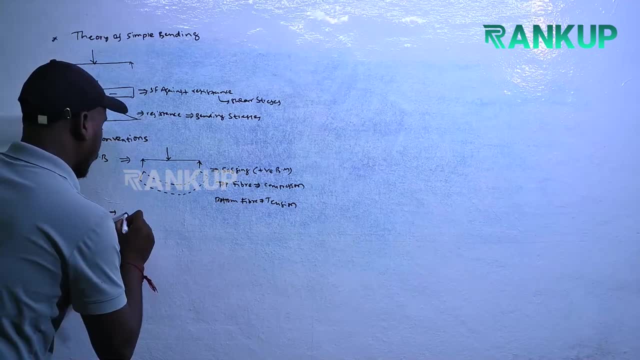 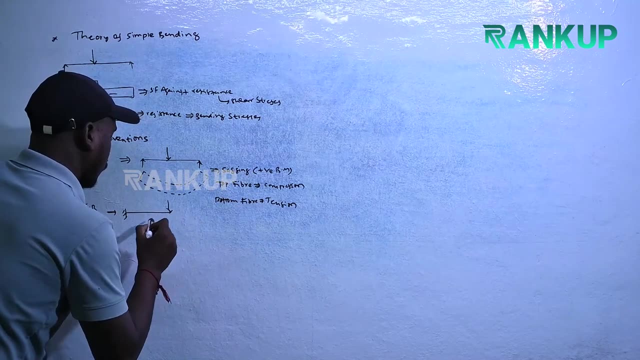 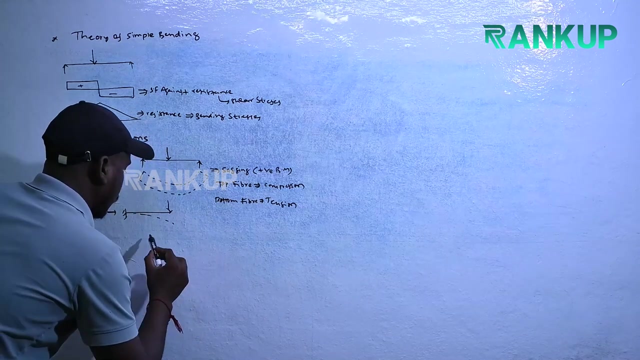 For the cantilever beam. For the cantilever beam, we take it like this, It will hog. If we take a load, it will hog. What is the hogging here? For example, if it comes like this, it will come like this. 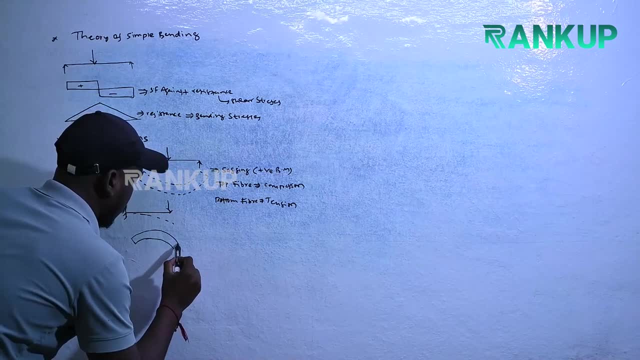 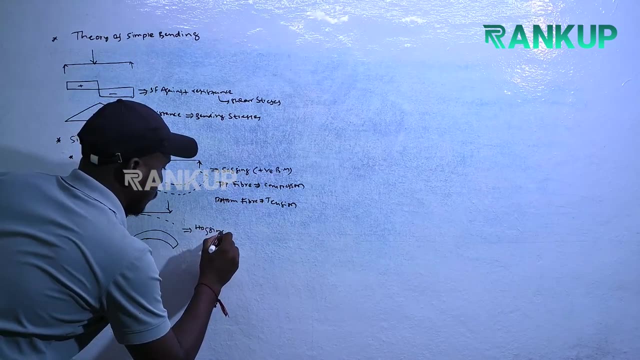 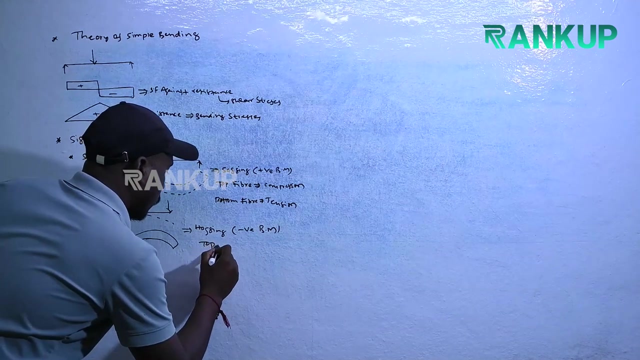 This is the hogging, This is the hogging. This is the hogging In this. what is the hogging? What is the hogging? We said negative bending moment. Negative bending moment. What happens to the top in the hogging? 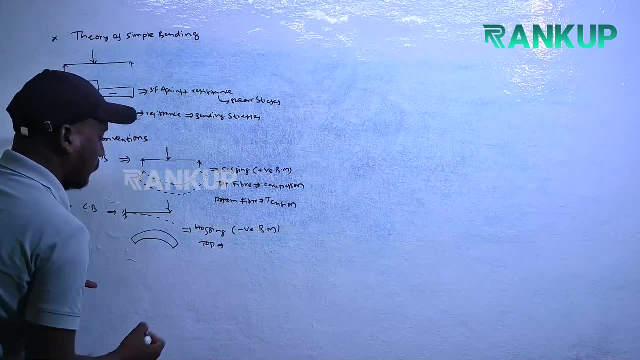 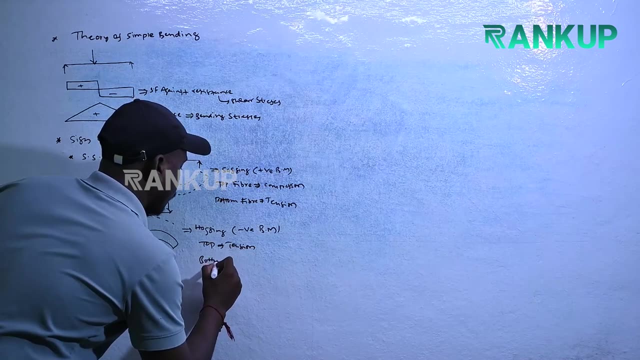 What happens to the top fiber? Top fiber is the top layer. What happens to the top fiber? It is in tension. What happens to the bottom fiber? What happens to the bottom fiber? It is in compression. What happens to the bottom fiber? 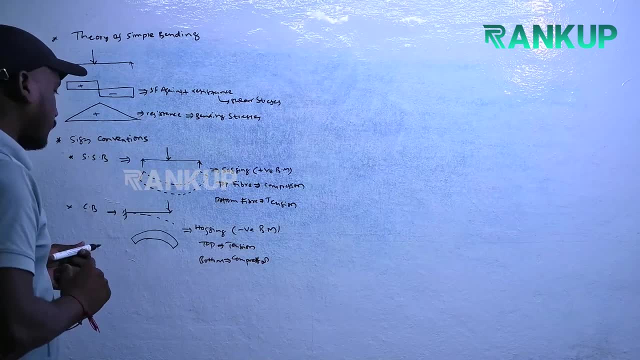 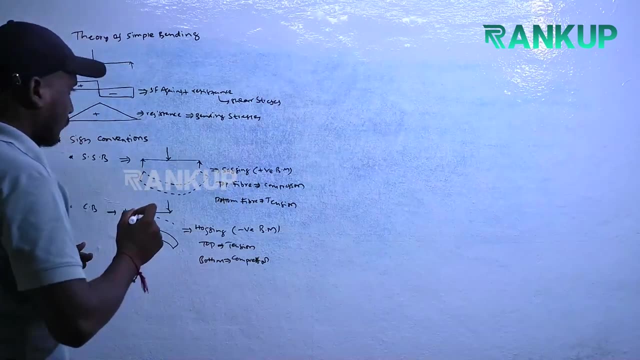 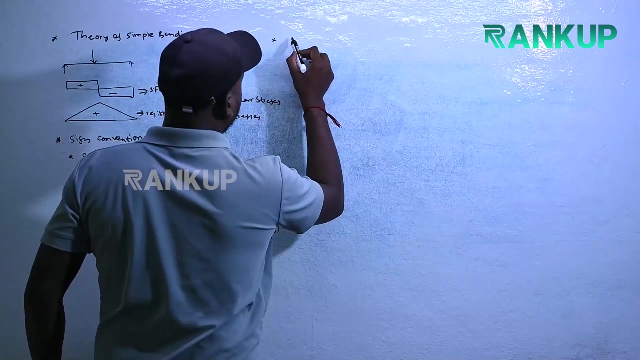 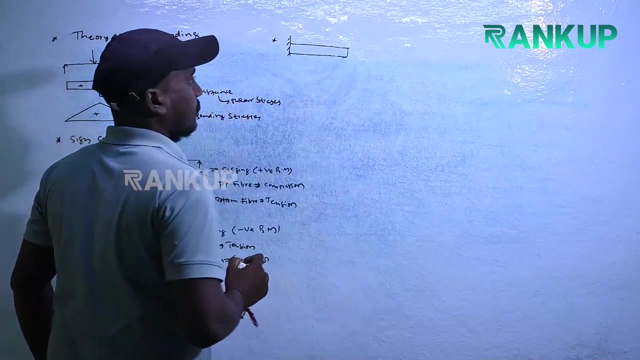 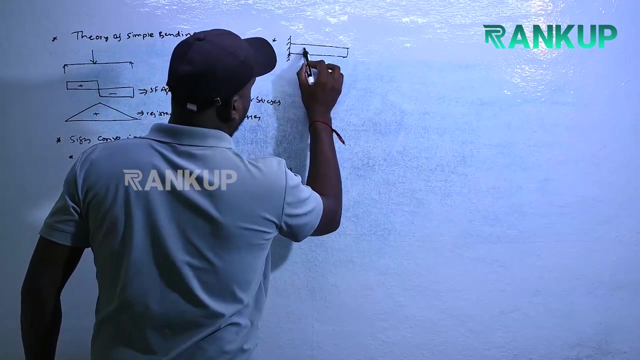 It is in compression. Ok, This is the sign convention. This is the sign convention For this. what happens next is: this is a beam, For example. this is the beam. what happens near this beam is: all these layers are there. what happens near this beam layer is: 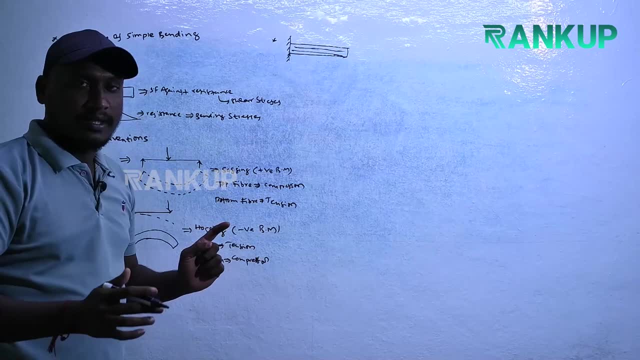 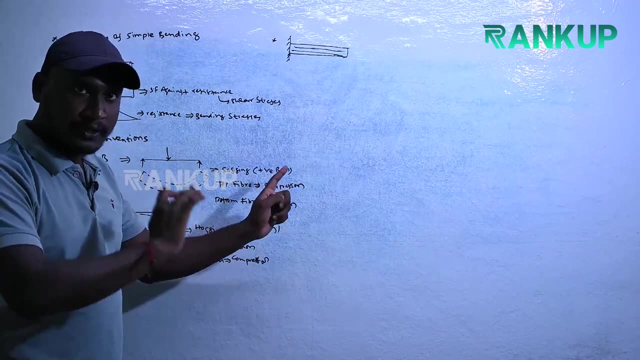 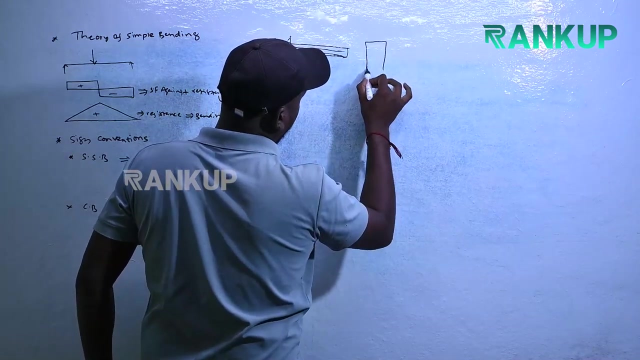 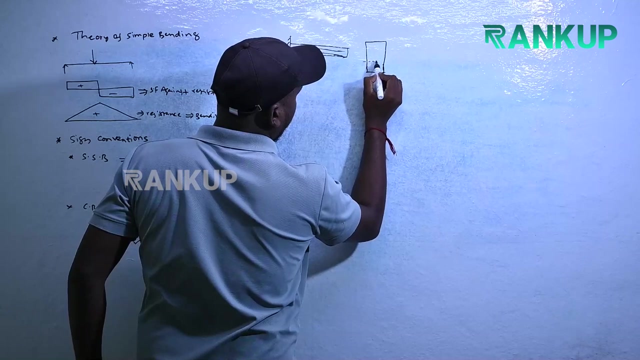 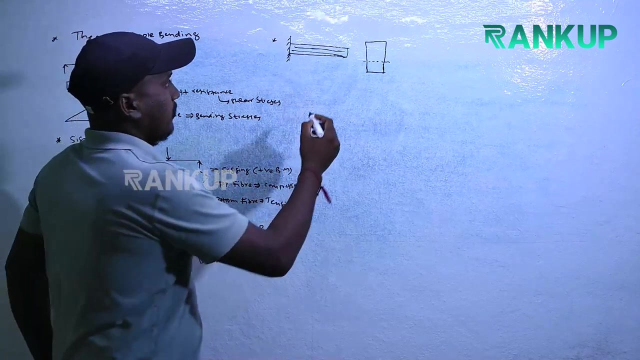 near one layer, there is no stresses or strain developed at a layer. that layer is called neutral layer. the cross section of this beam is a rectangle, so the neutral layer intersects the intersection of the neutral layer with the cross section of the plane. the intersection of the layer is known as neutral axis. 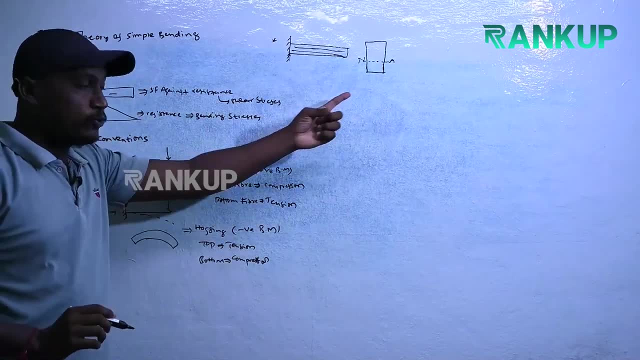 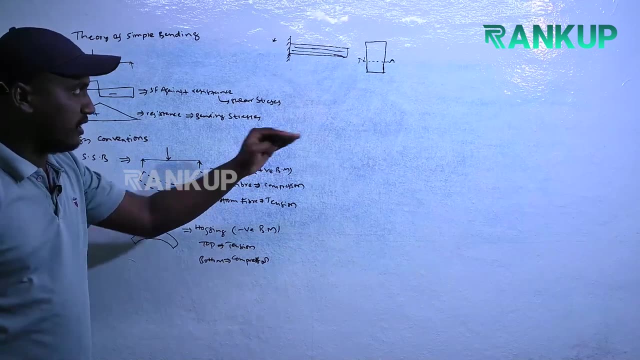 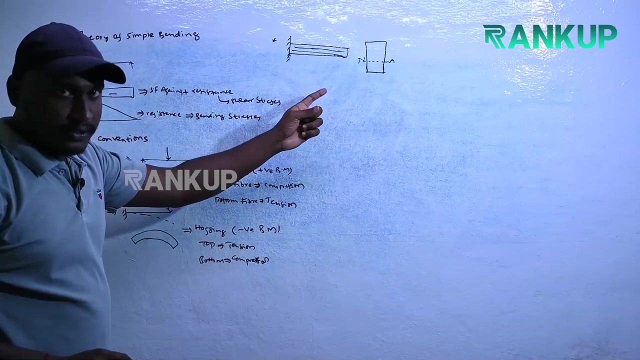 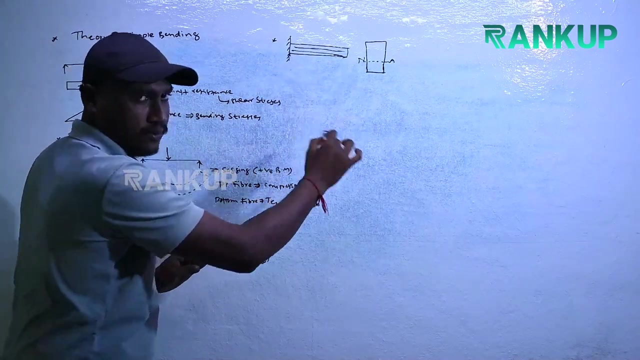 we call it neutral axis with the cross section. what happens here is there is no stresses or strain developed at that point, at that section, at that layer. we have to observe this: what is the first neutral axis? first, a beam is comprised of many number of layers. number of layers: 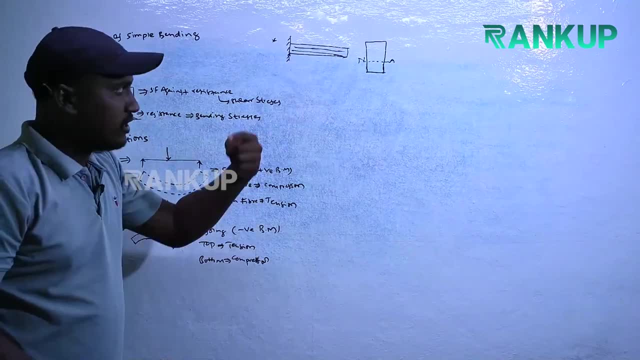 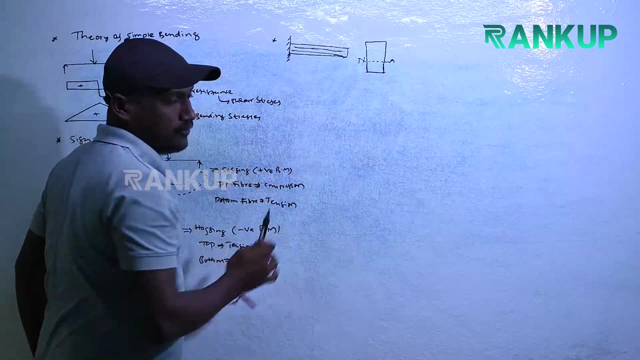 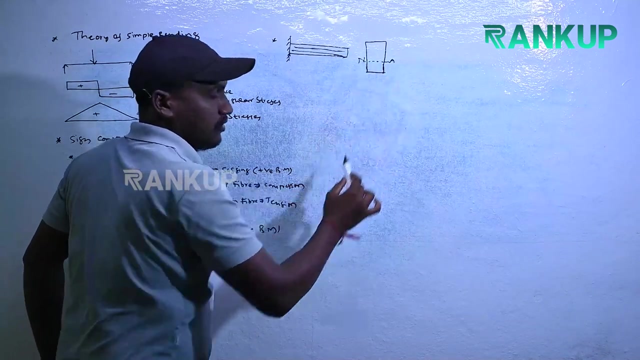 what happens here is there is no stresses or strain developed at a layer. that layer intersects with the cross section of the plane of that beam. that intersection of the cross section is known as neutral axis. we call it neutral axis. that is the definition for the neutral axis. 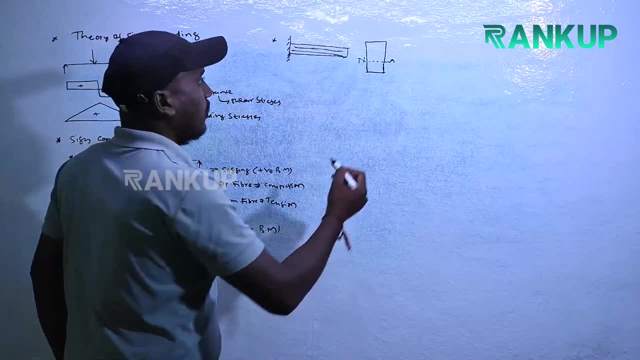 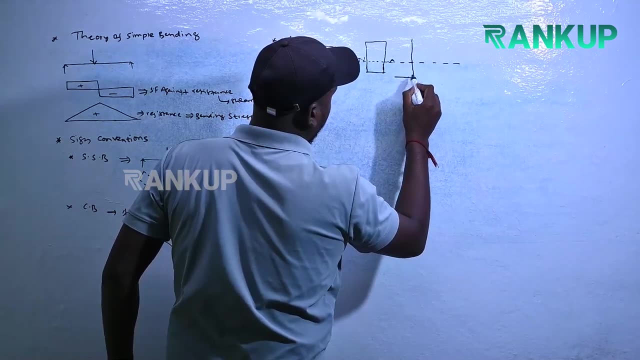 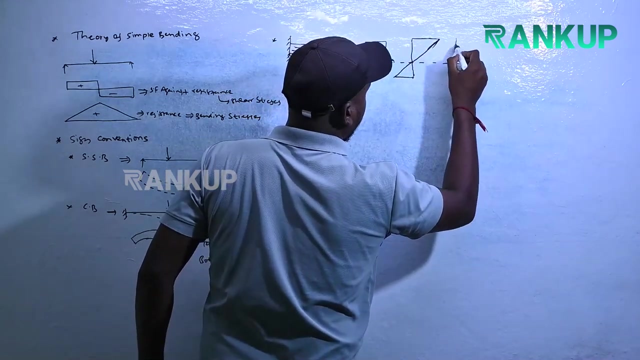 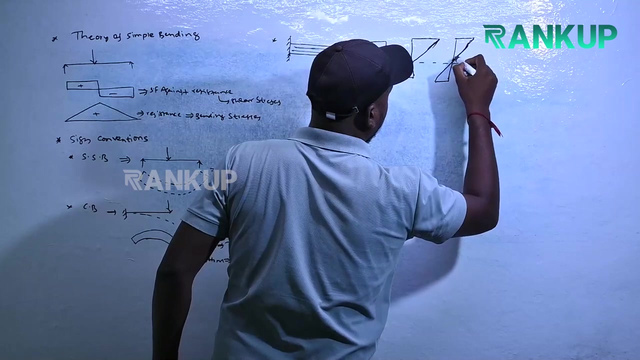 what happens near the neutral axis? there is no stresses or strain developed. I am drawing a stress-strain diagram for this cross section. how it comes. how it comes. how it comes- ok, sorry, how it comes. stress-strain diagrams: ok, stress-strain diagrams- how it comes. 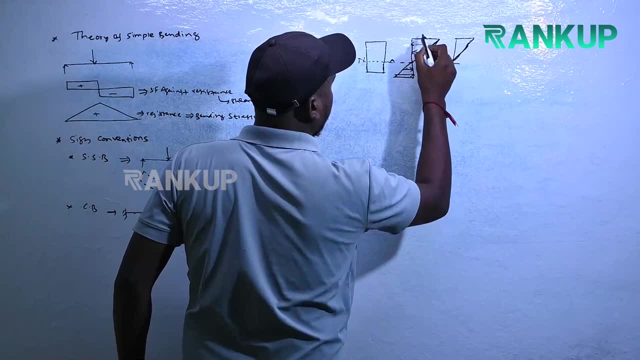 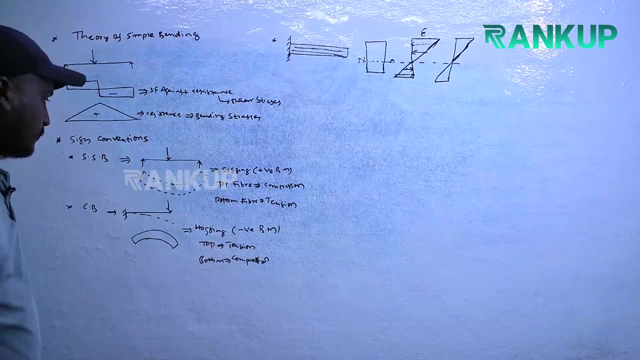 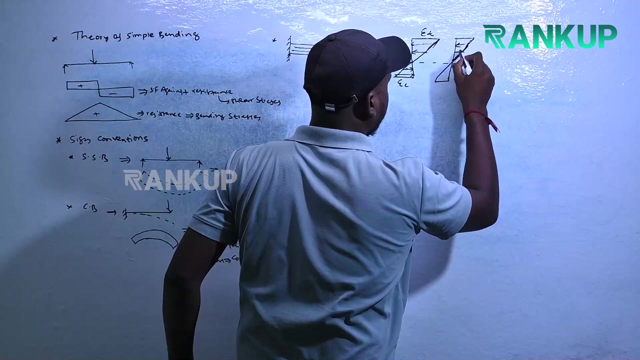 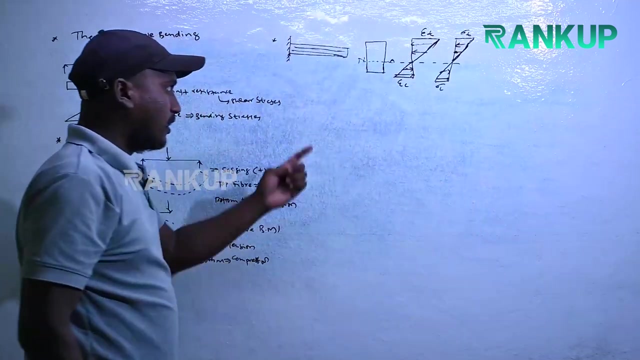 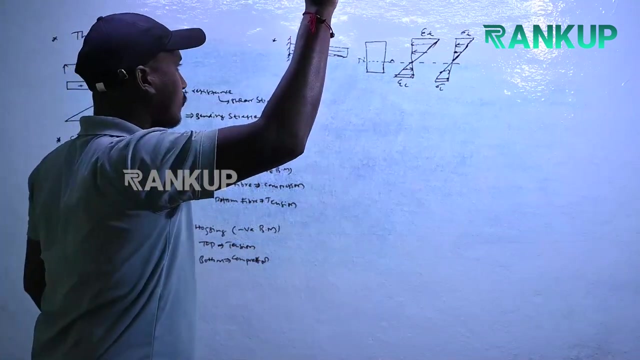 sorry, ok. ok, this is epsilon. this is cantilever beam. what is above, above is tension, below is compression. this is stress diagram. ok, stress diagram is sigma t, sigma c: ok, this is the stress-strain diagram. ok, near neutral axis: we have zero. near neutral axis, we have zero. 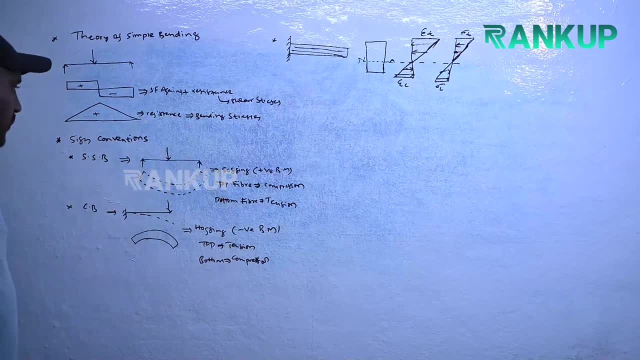 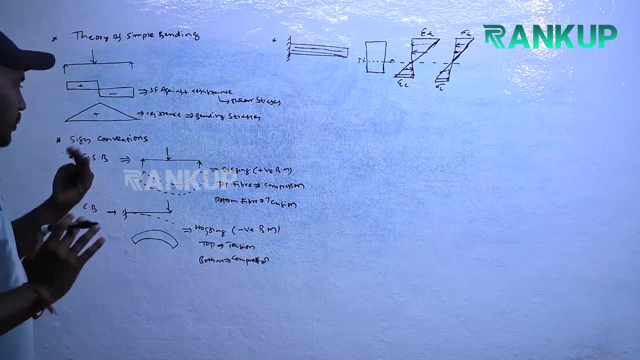 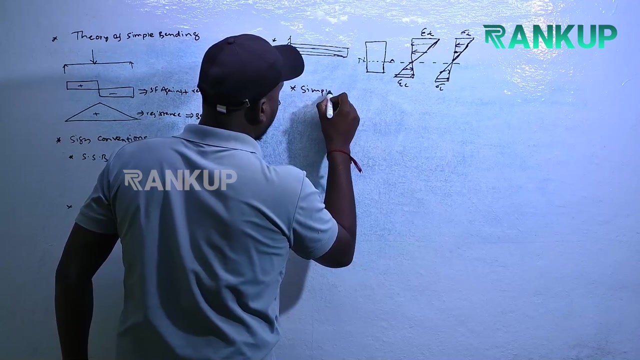 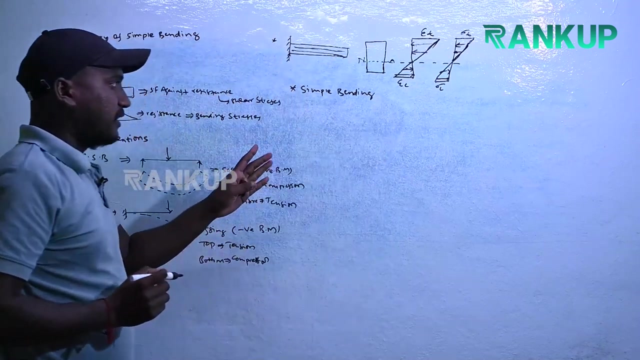 ok, that is basic concept, that is sign convention basic concept. ok, in case of cantilever, in case of simply supported beam. ok, that is it. so, in case of simple bending, what is simple bending next is: what is simple bend? ok, simple bending. so what is simple bending? 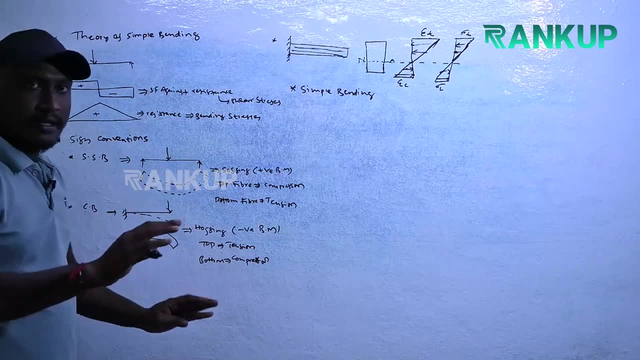 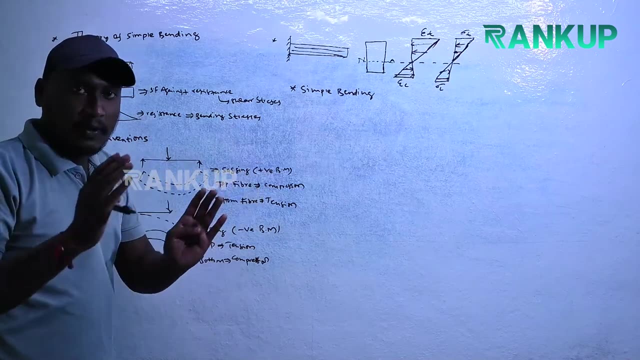 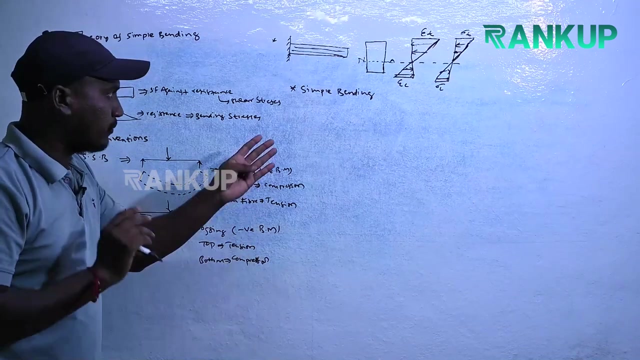 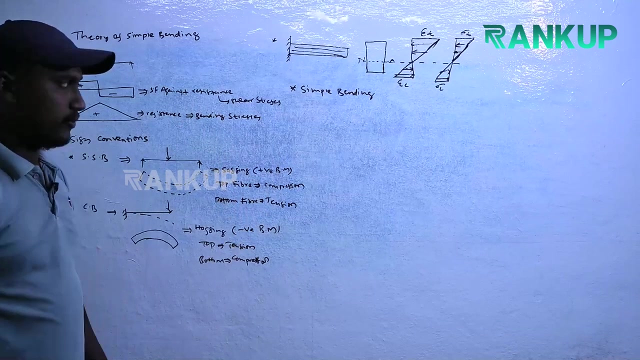 on a beam. a beam is bend only due to the bending. ok, the bending of a beam is due to uniform bending moment force acting on the beam. There is no shear force acting on the beam. The type of bending is known as simple bending. We call that simple bending. For example, I am taking cantilever beam. 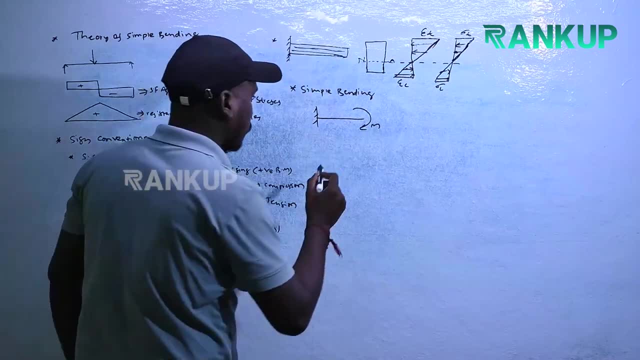 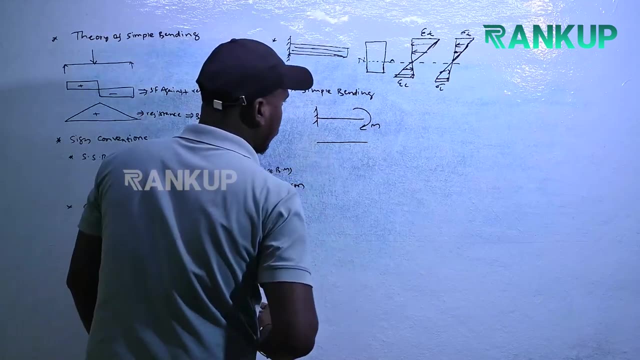 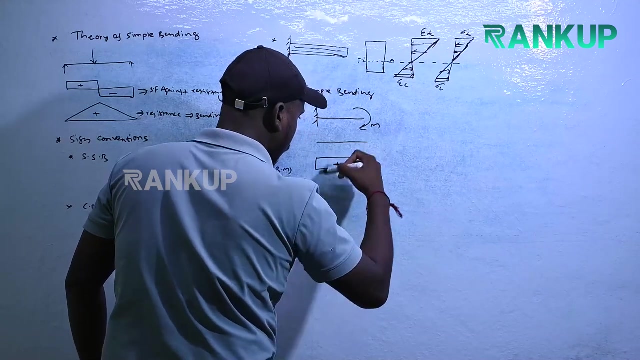 subjected with momentum at the free end. So what happens to the shear force diagram? The line comes: There is no shear force generated in the cantilever In case, if we take the bending diagram, it is uniform bending moment. It is negative, It has to be negative Here, in simple. 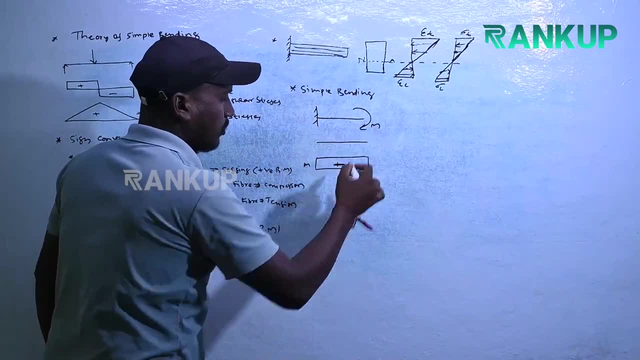 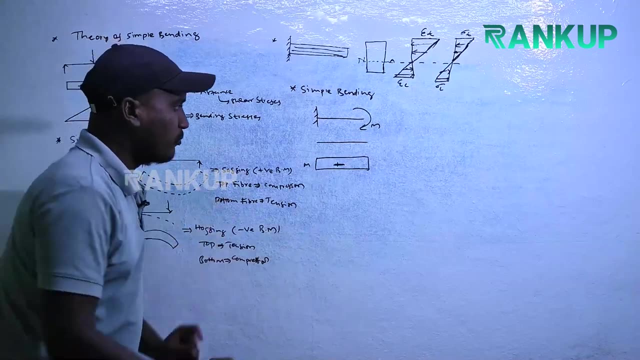 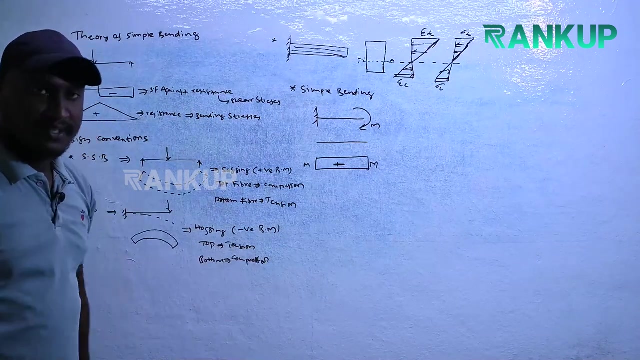 bending when the cantilever beam acts on the moment, at the free end. there is no shear force in this bending, in this beam, Only moment is there, Only uniform moment is acting. We call that simple bending. We call that simple bending. What is simple bending? There is. 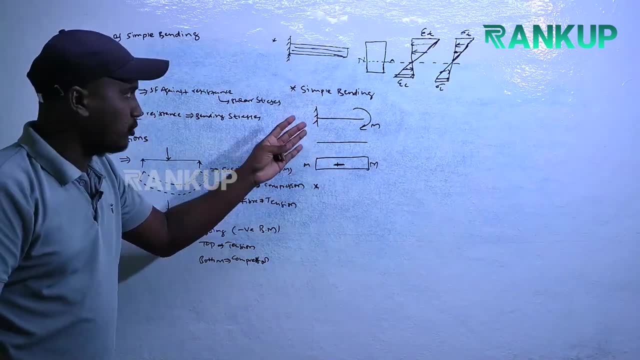 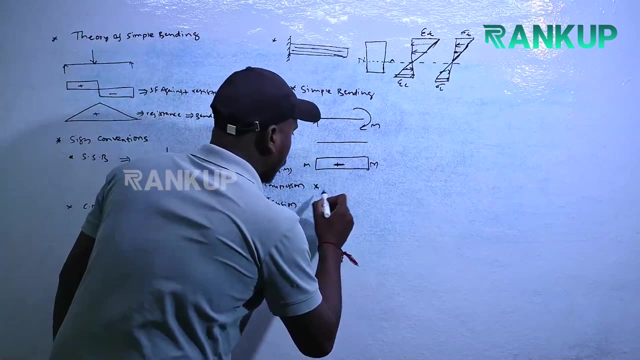 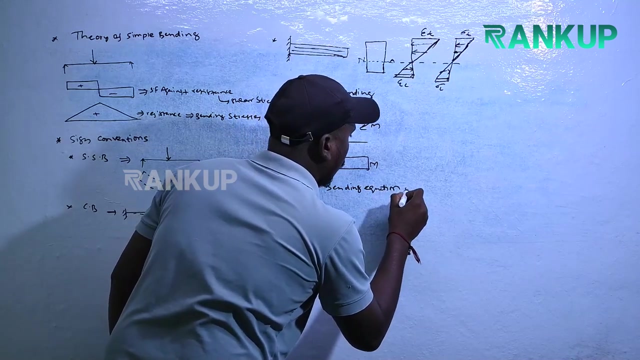 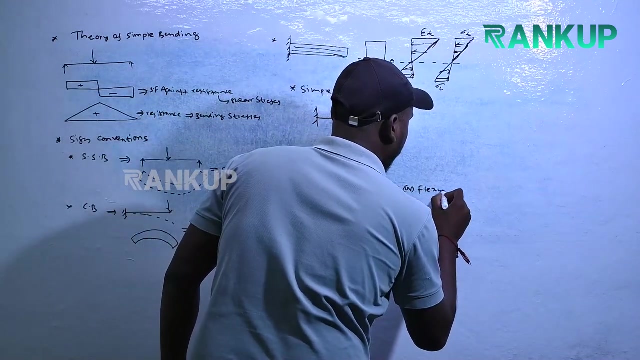 no shear stress. Only the beam bends due to the bending moment. Okay, That is simple bending. That is simple bending. Next, we have bending equation. Next we have bending equation, or bending equation, or flexural equation, Or flexural equation. Okay, This bending equation, or 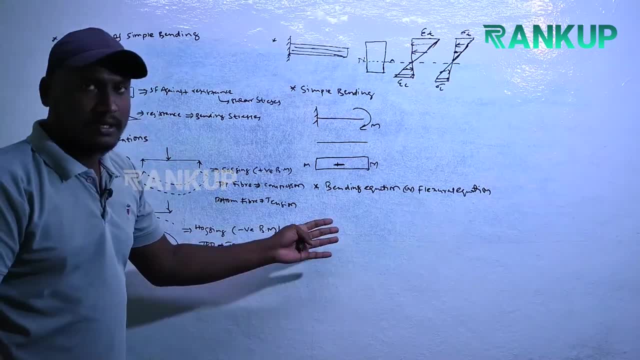 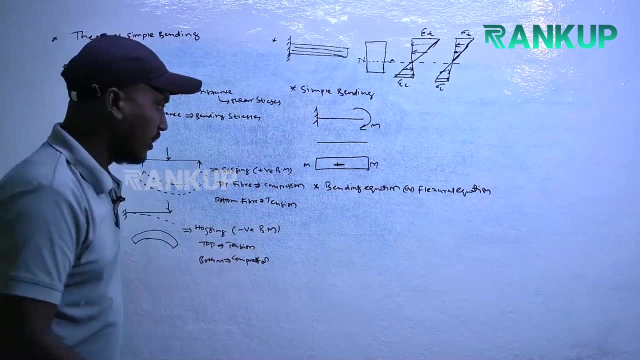 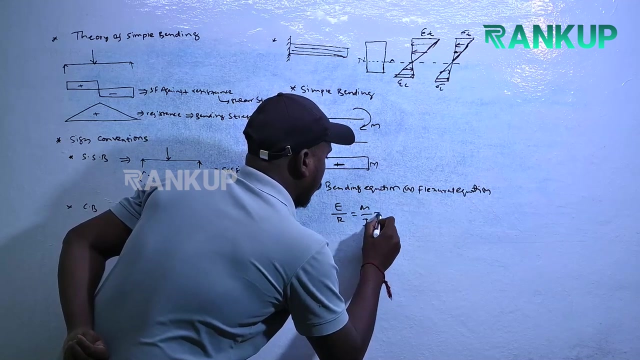 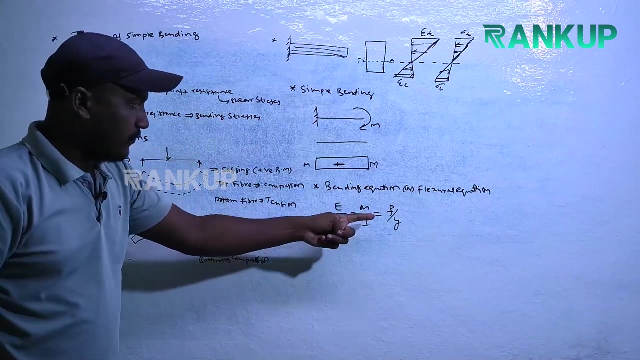 flexural equation, or derivation, does not need to be present now, because there is no derivation at the diploma level. We have only the equation. Okay, How to remember this equation? How to remember this equation, Elizabeth Rani, may I follow you? May I follow you, Elizabeth Rani? may I? 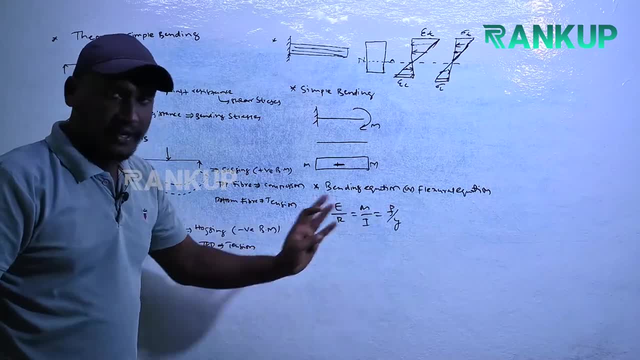 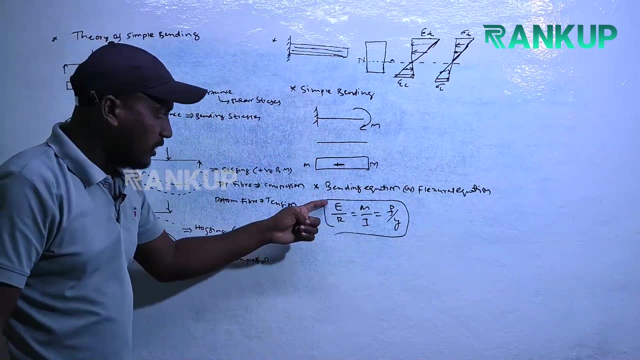 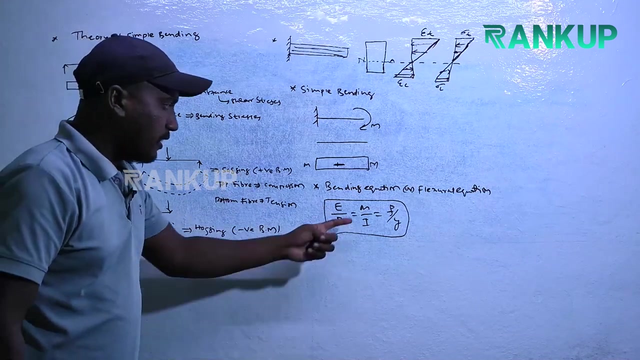 follow you. Okay. E R M I F? Y. Okay, Now let us go to the subject. What is E? You know. please write down What is E. It is Young's modulus of the material. Capital R is radius of the curvature. Capital M is: 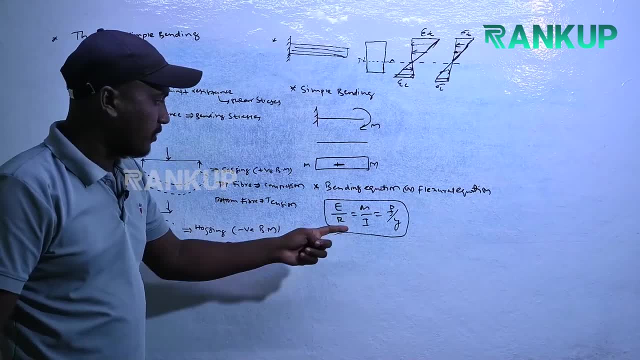 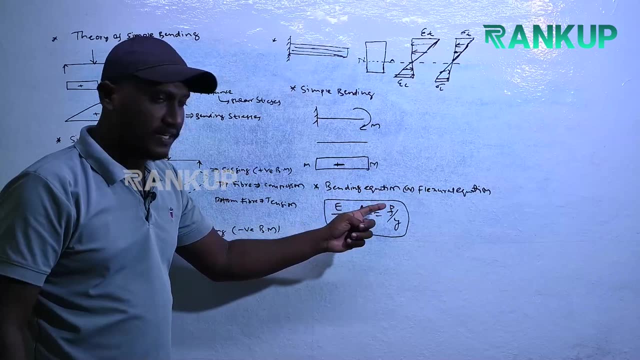 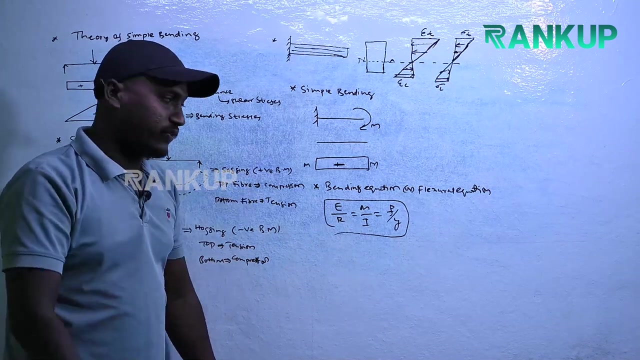 moment of resistance or bending moment. I is moment of inertia. F is bending, bending stresses or flexural stresses. Y is small. y is distance from the neutral axis to the outermost fiber. Distance from the neutral axis to the outermost fiber To the outermost. 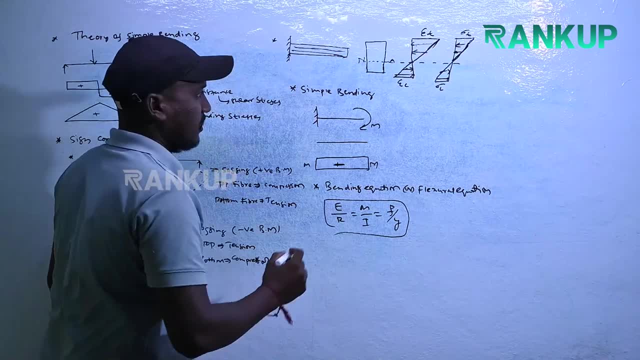 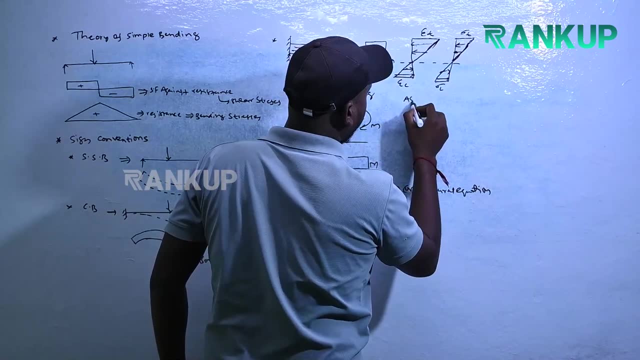 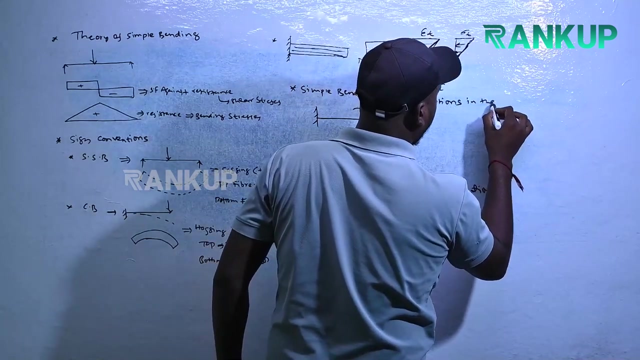 fiber. Okay, Next assumptions. Next, we have assumptions in assumptions. You can write them. Okay, Now dictate here. Just highlight points. You can write assumptions in theory of simple bending, In theory of simple bending, Theory of simple bending. 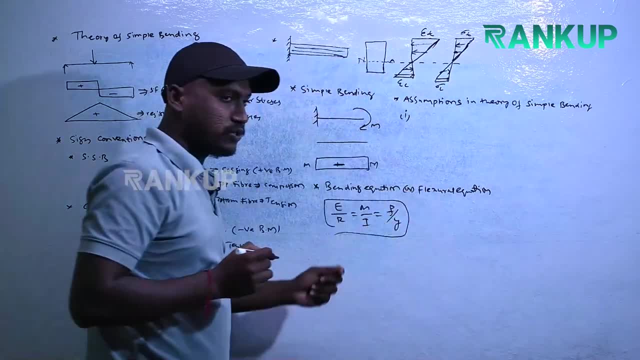 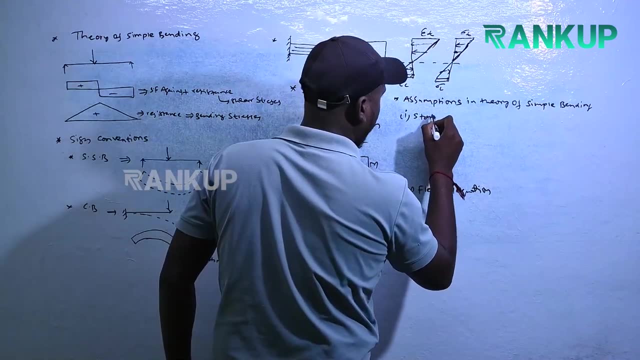 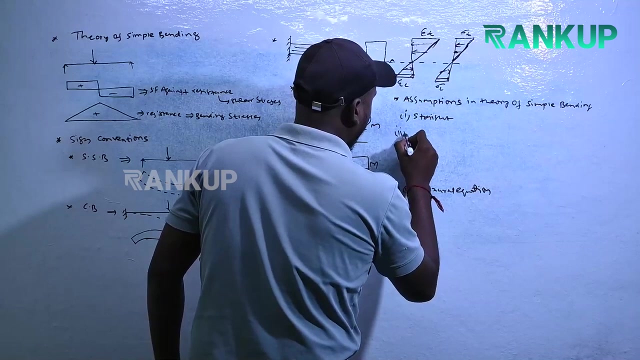 Okay, First assumption. First assumption, which is: the beem is initially. the beem is straight Initially, beem is straight Initially, beem is straight. Please write down: Initially the beem is straight. Second second, which is the second, which is the material Material: 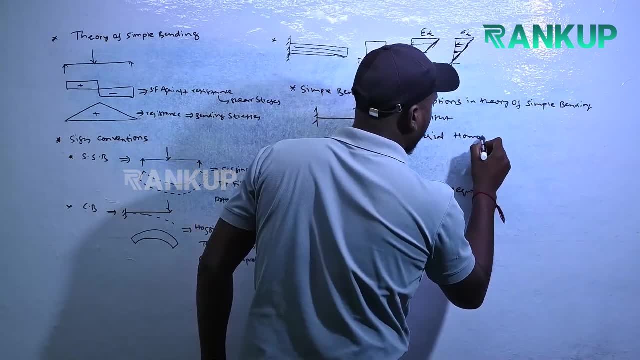 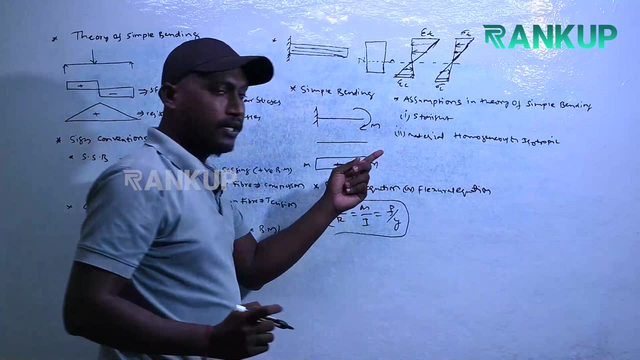 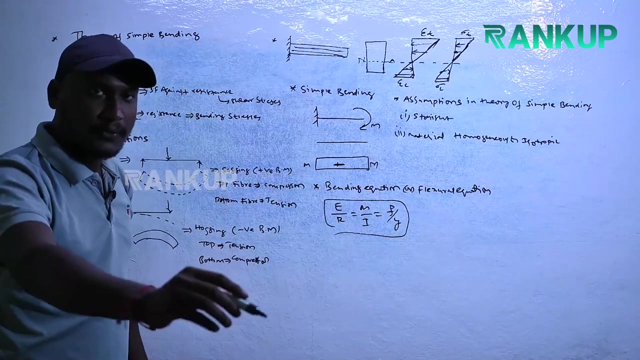 of the beem is homogeneous and isotropic, Homogeneous and isotropic, Homogeneous and isotropic. second point: in the material of the beam is homogeneous and isotropic. already you know: homogeneous, and at all points in a given direction the properties are same. okay, now the 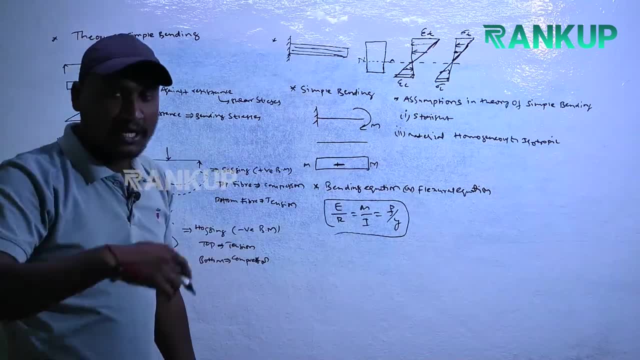 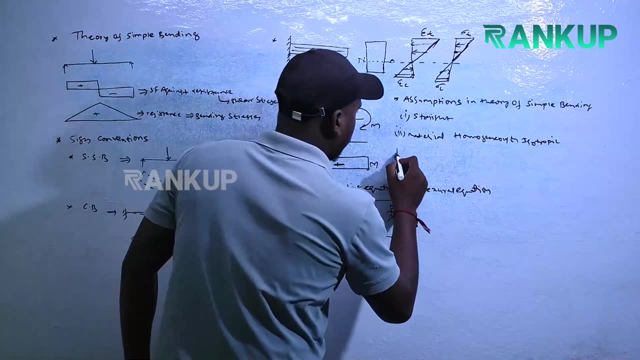 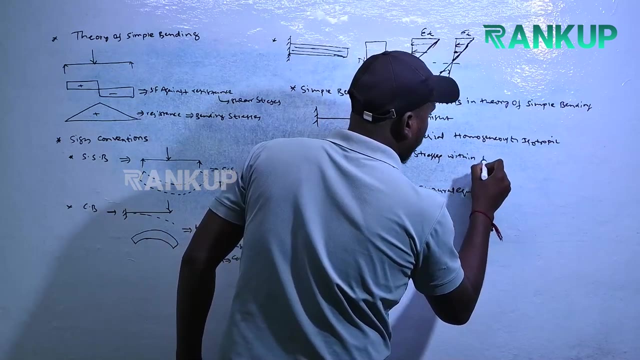 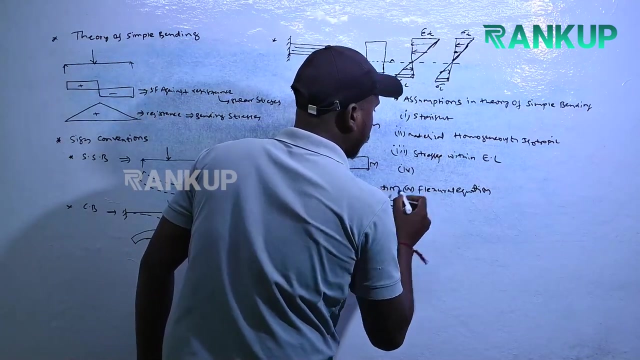 homogeneous isotropic and at a point, in all directions the properties are same. the isotropic, okay, material and homogeneous isotropic. next to third one: stresses are within stresses or within elastic limit. okay, now, stresses are within elastic limit. next, fourth, fourth point is very, very important point, that is, transfer sections. 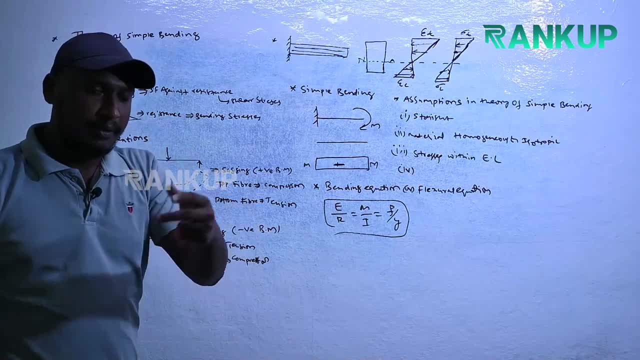 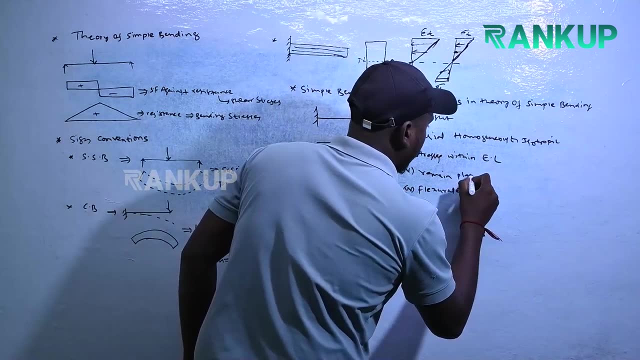 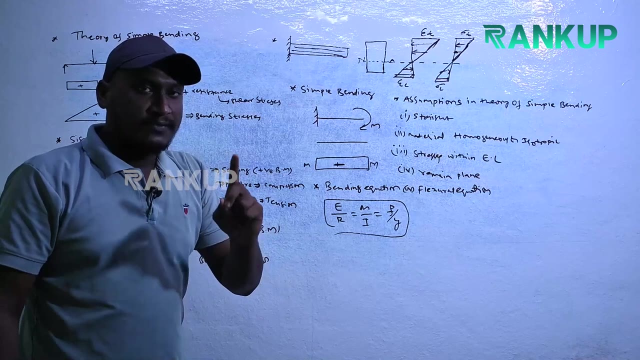 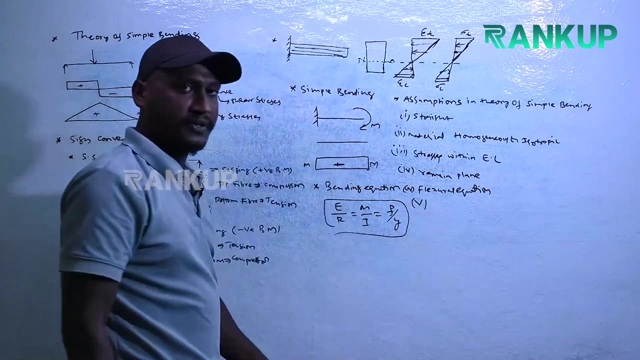 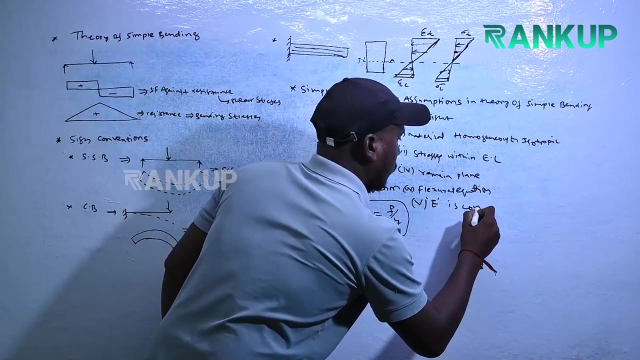 plane before bending, plane before bending. remain. plane after bending. okay, now remain plane. remain plane before and after bending. okay, now transfer section, fourth point. please write down fourth point: transfer sections remain plane before bending and after bending. next fifth point, next fifth point. fifth point is: modulus of elasticity is constant. modulus of elasticity is constant in compression. 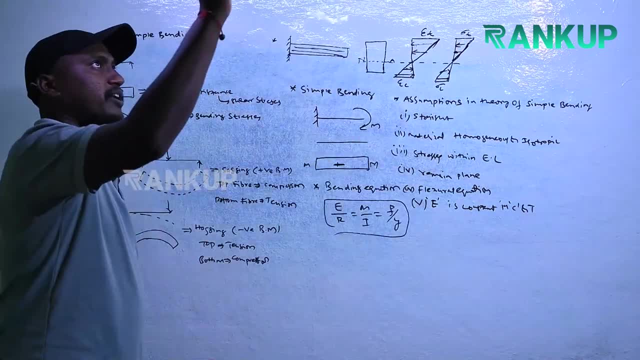 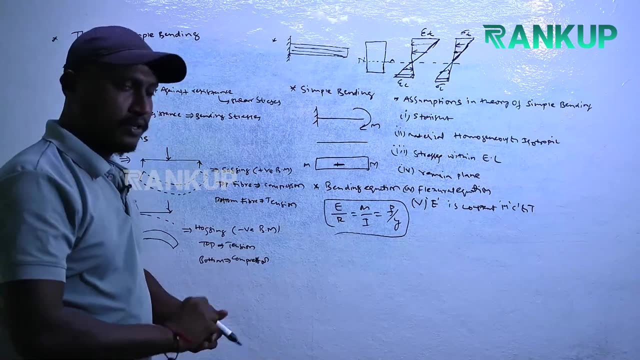 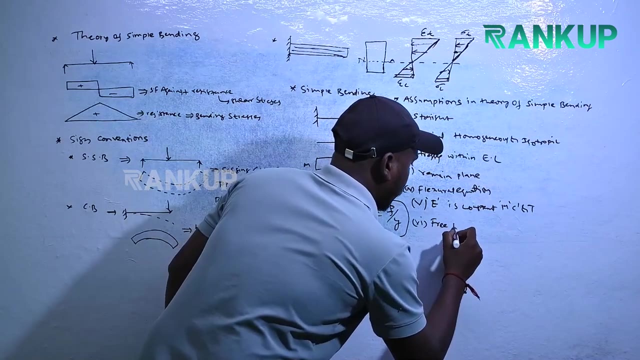 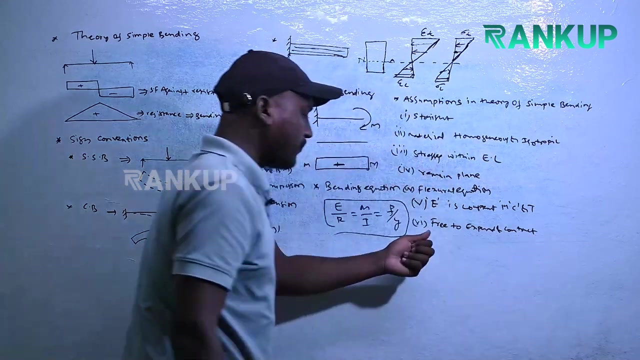 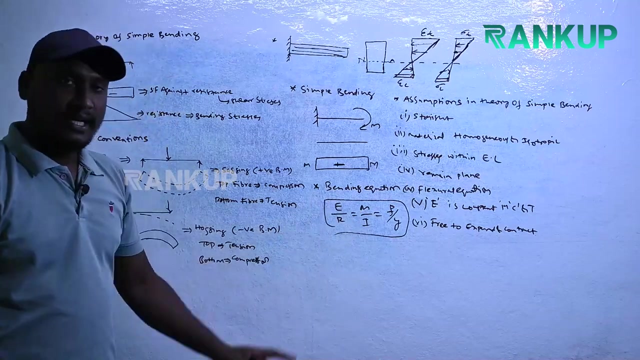 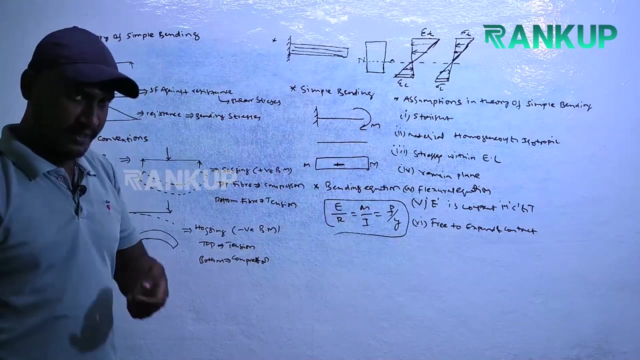 and tension in compression and tension. okay now, modulus of elasticity is constant, always in compression and tension. Okay now, next sixth point. Sixth point is free to expand and contract. Free to expand and contract, And each layer of the beam, each layer of the beam, is free to expand and contract. That is the sixth point. That is the sixth point. These are some of the. these are the assumptions of the simple bending theory. Simple bending theory. 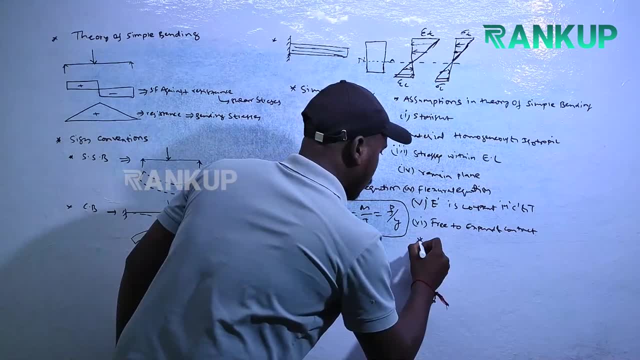 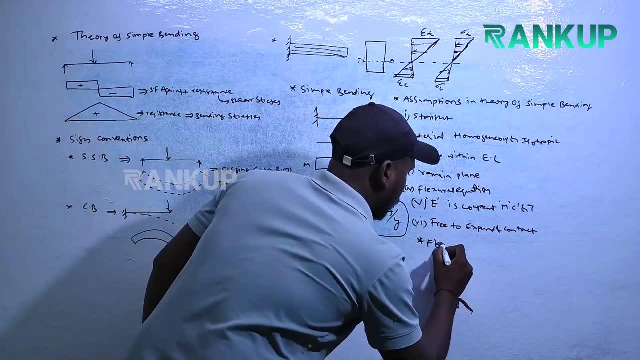 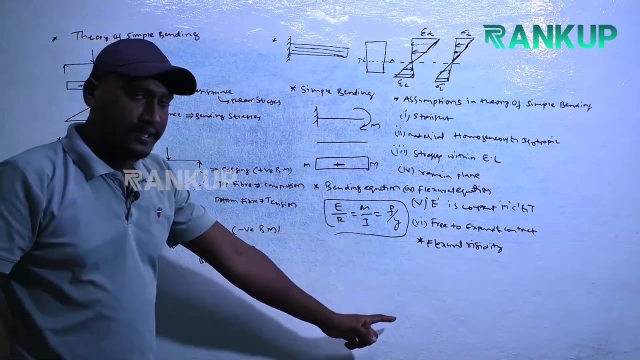 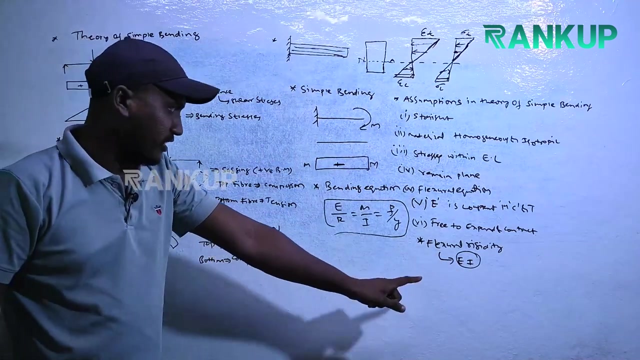 Then we have. then we have flexural rigidity and flexural rigidity. Keep it as a flexural rigidity. New topic, that is flexural rigidity. Okay now flexural rigidity, Flexural rigidity and it is the product of the modulus of elasticity and moment of inertia. We have already discussed many times here also there, flexural rigidity and the product of the modulus of inertia. 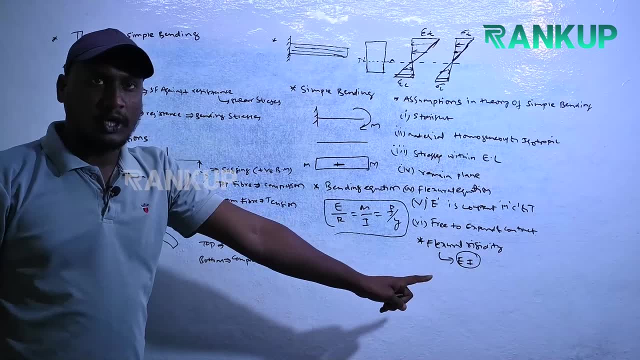 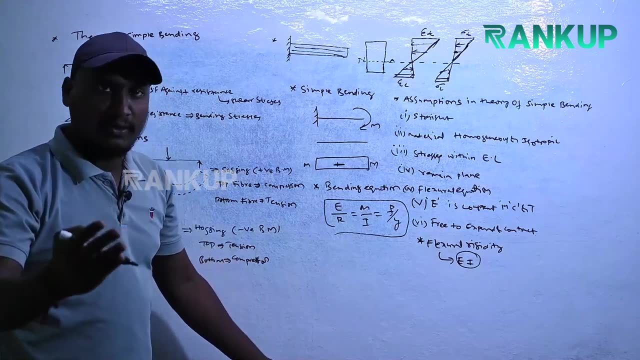 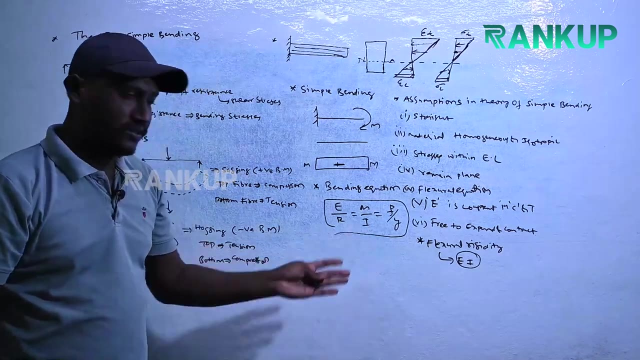 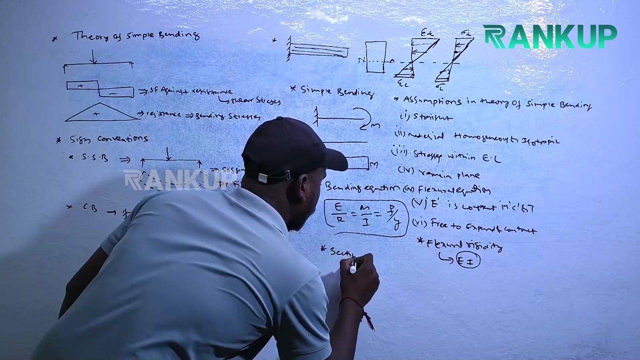 The modulus of velocity of the material and the moment of inertia of the cross section. Okay, That is what we call flexural rigidity. Flexural rigidity is strong. As the flexibility increases, the strength of the member will also increases. Okay, That is flexural rigidity. Next we have, next we have, section modulus, or modulus of section, Section modulus. 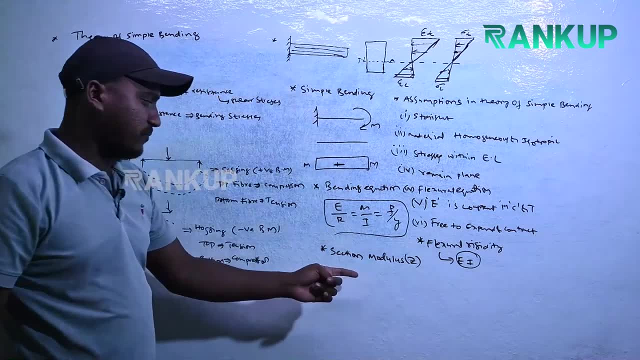 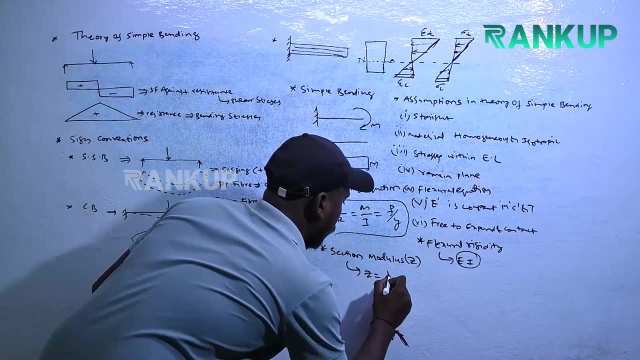 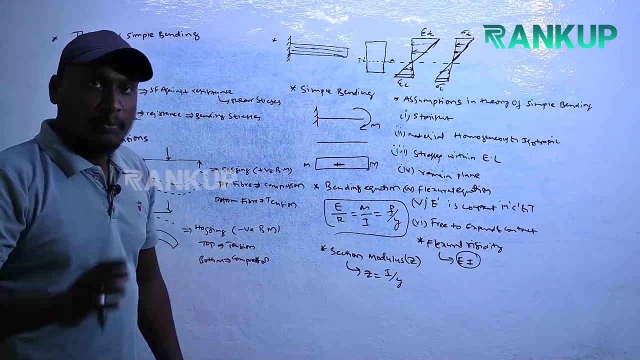 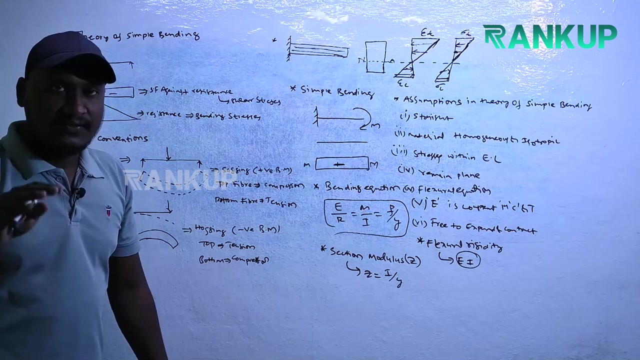 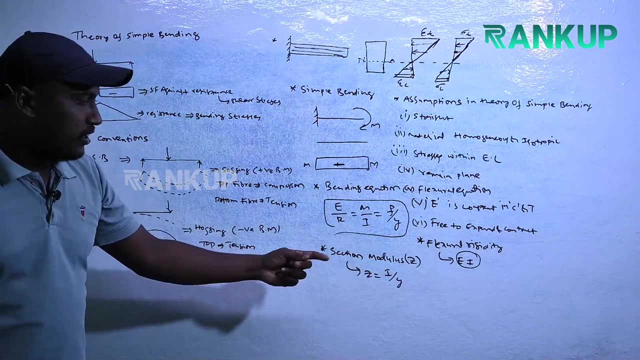 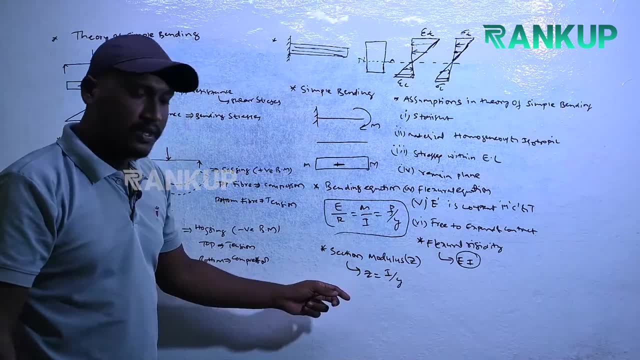 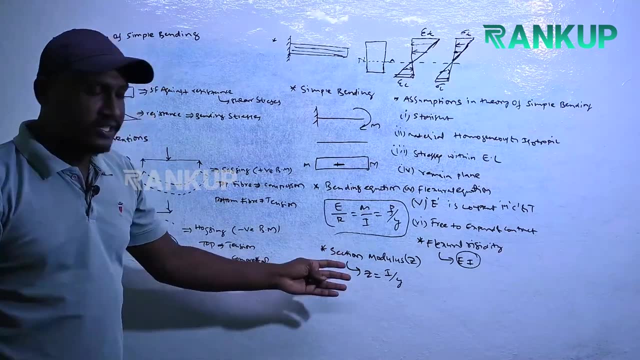 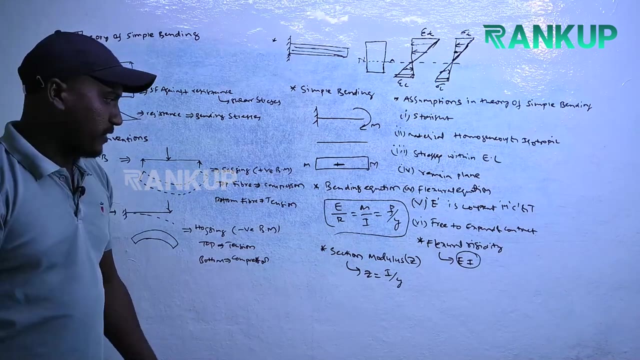 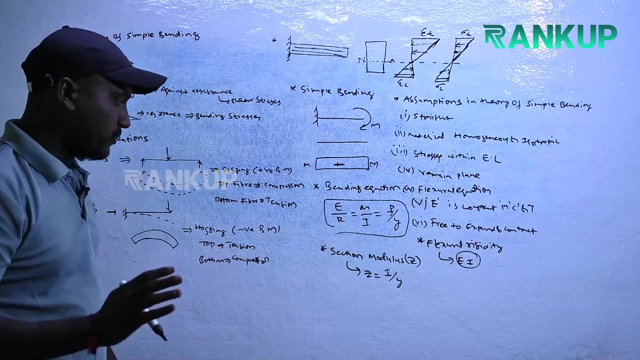 We will indicate section modulus with z. we will represent section modulus with z. once again, section modulus is very, very important. section modulus means it is the ratio between the moment of inertia to the distance from the neutral axis to the outermost fiber. that is what we call section modulus. we need to write some standard geometrical, standard geometry. we will write section modulus. first we will say rectangle. 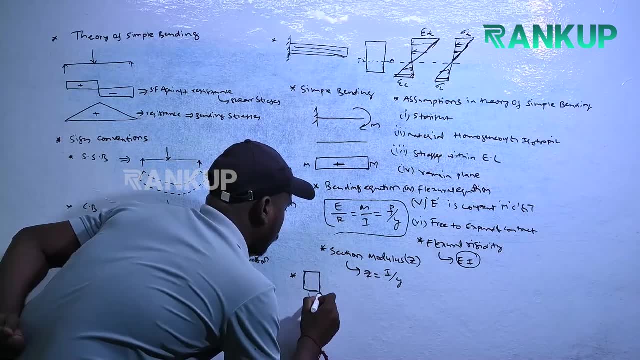 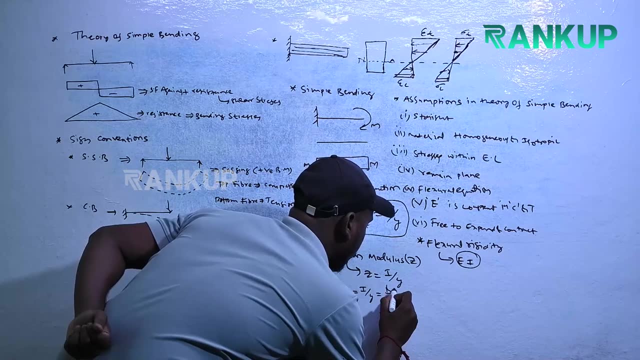 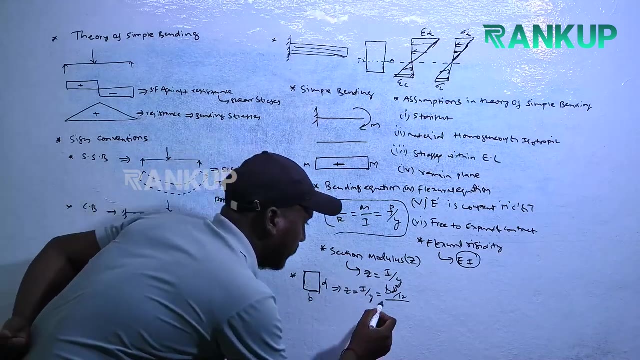 first we will say rectangle. rectangle width b, depth d, section. modulus is: z is equal to i by y. moment of inertia for the rectangle is bd cube by 12, divided by y is the outermost fiber from the neutral axis, that is d by 2,. keep one thing in mind: for standard geometries, neutral axis is passed from the center. 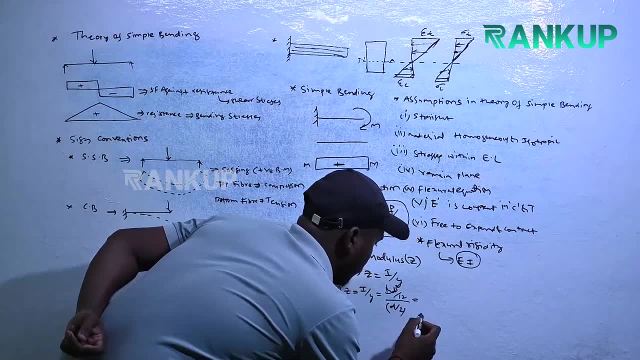 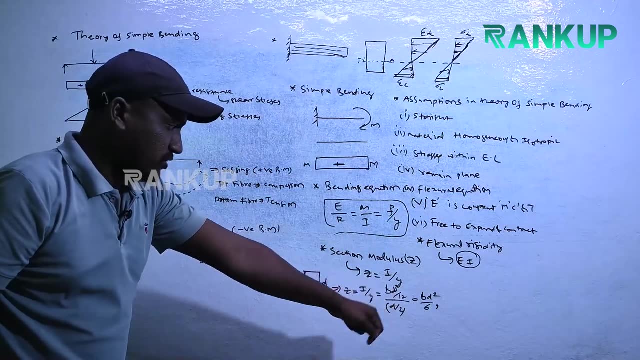 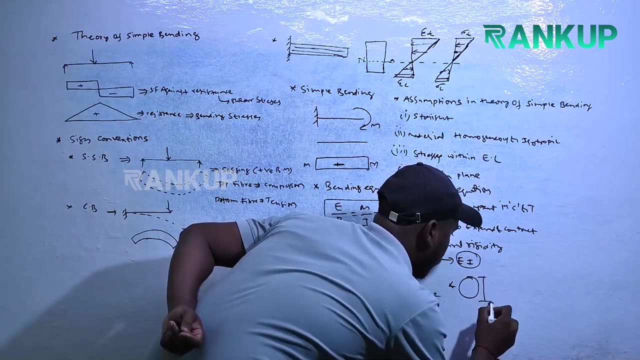 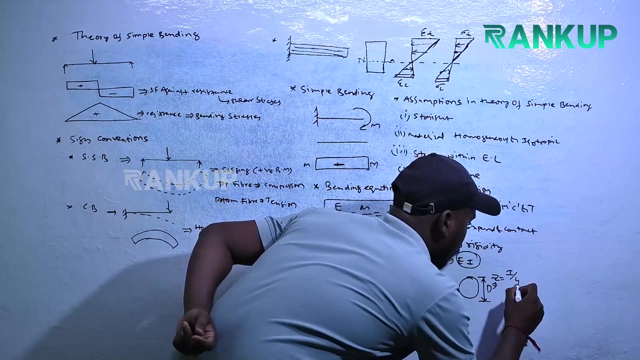 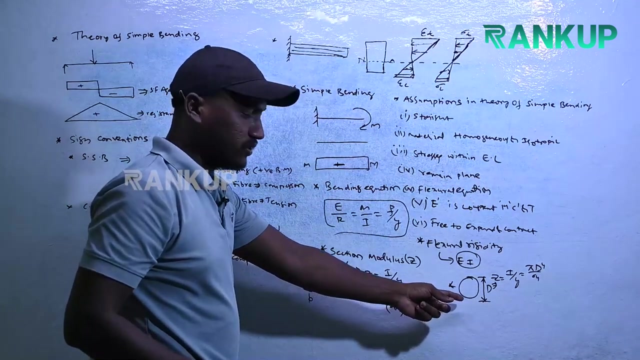 okay, now then bd cube by 12, divided by d by 2, then what will happen to us? bd square by 6 will come. that means d cancel will come b2, 2, 1,, 2, 6, bd square by 6 for the rectangle, for the circular section: solid circular section. diameter capital D. okay, diameter capital D, then section modulus z is equal to moment of inertia by y, isn't it? 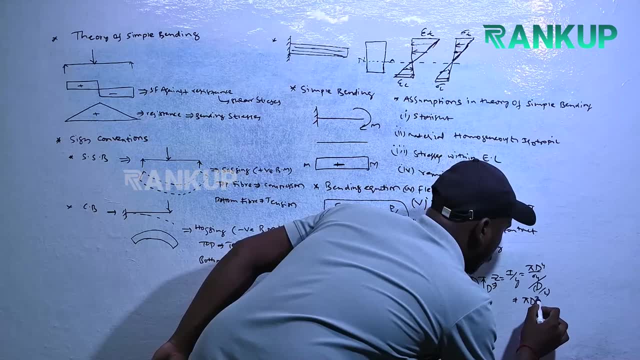 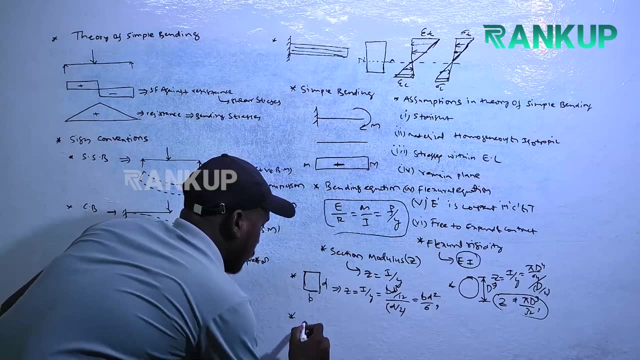 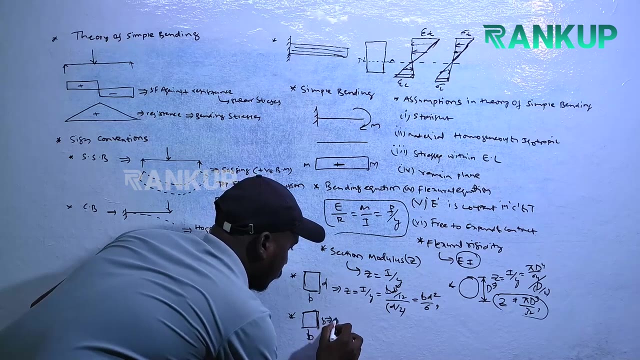 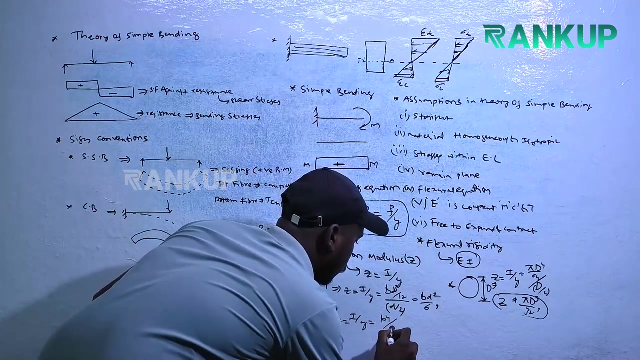 is d by 2.. Then we get pi d cube by 32.. Section modulus for the circular section. Next square is equal to i by y. i is b power 4 by 12 divided by b by 2.. Then b cube by 6.. For 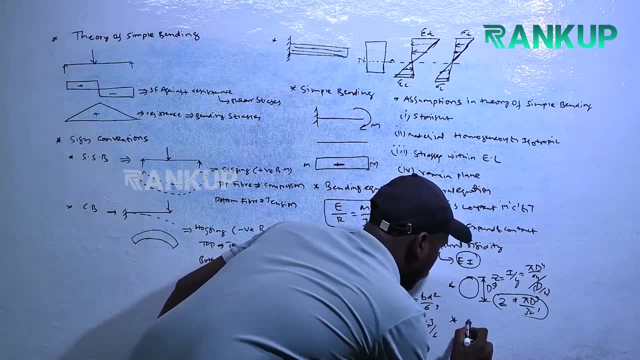 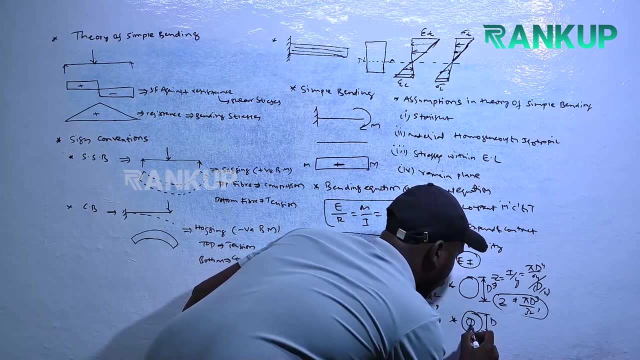 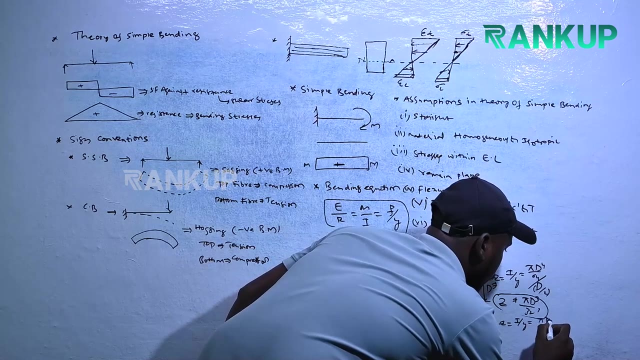 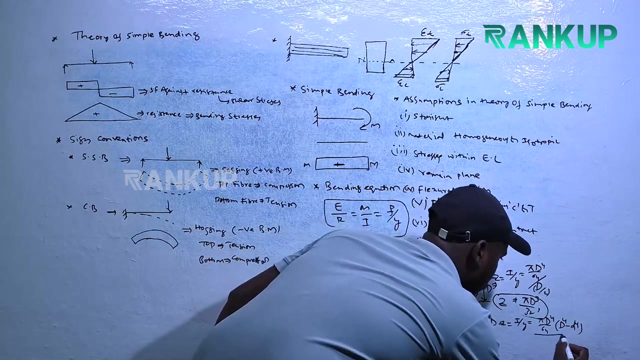 the square section, Next for halo circular. For halo circular: capital D, outer diameter and inner diameter, small d. Then z is equal to i by y. Then moment of inertia. is pi d power 4 by 64. whole d power 4 minus capital D power 4 minus small d power 4 divided by: 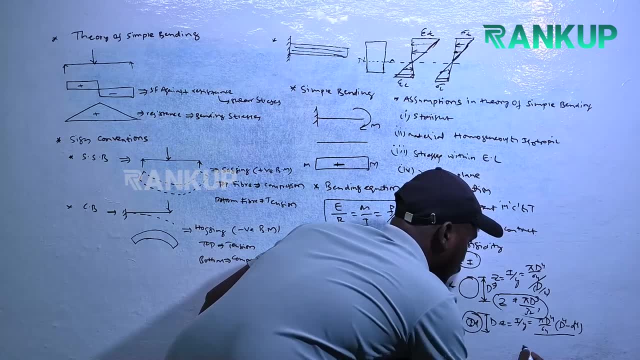 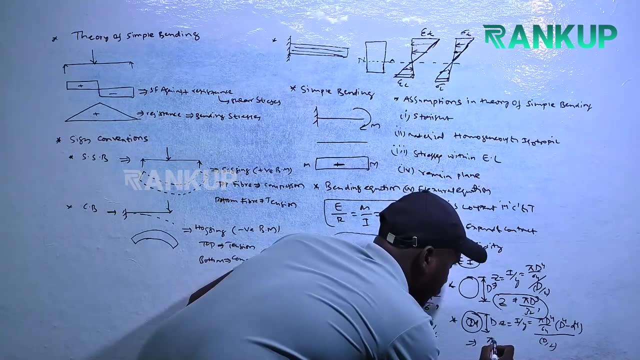 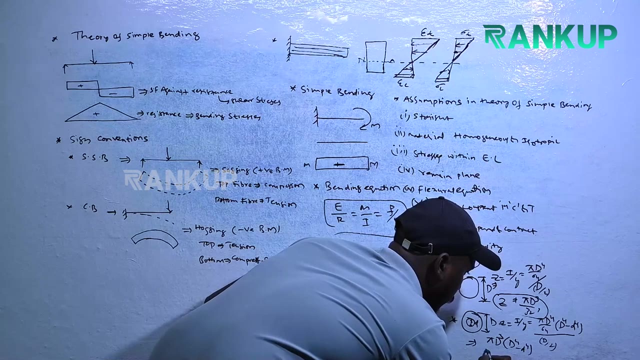 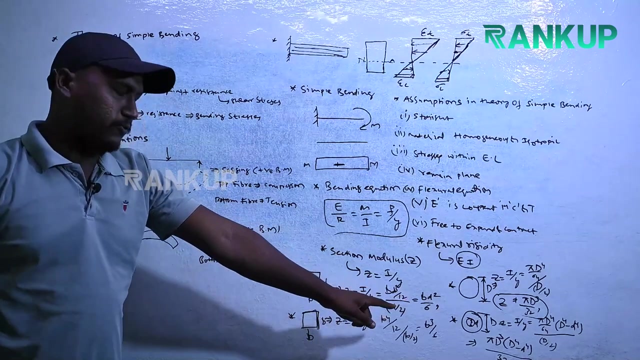 divided by What is y, y is capital D by 2.. So for halo circular, pi d cube into d power, 4 by small d power, 4 whole divided by 32.. Pi d cube by 32 into d power, 4 by d power, 4 minus capital D power. 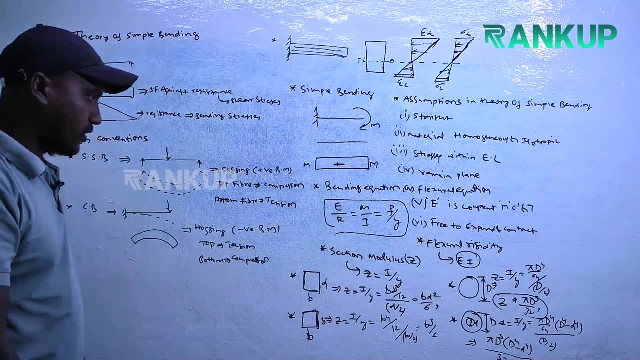 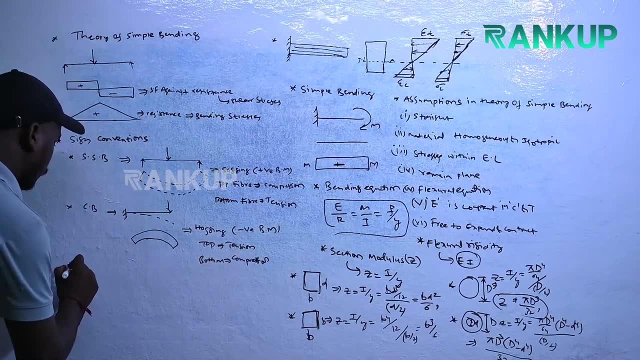 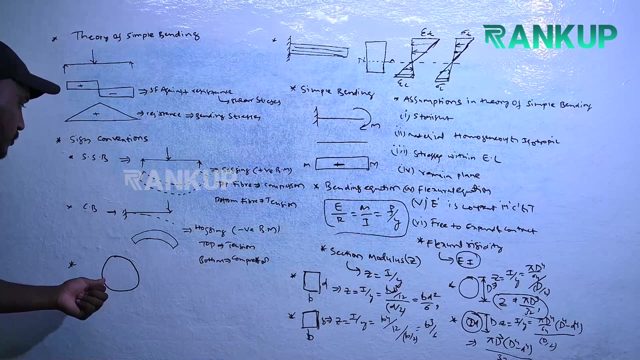 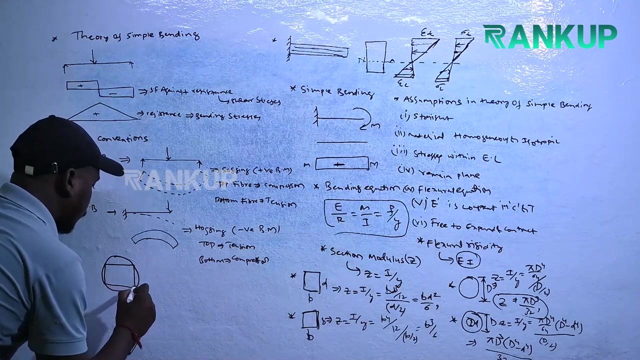 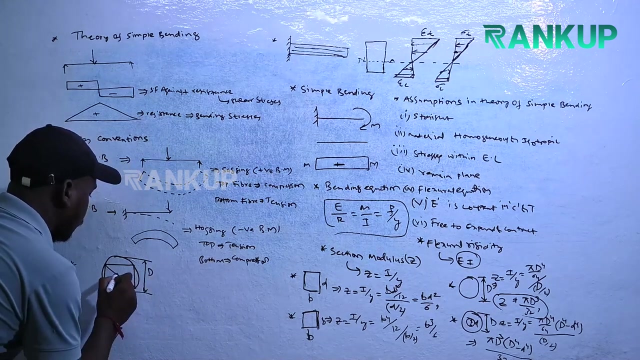 4 minus small d, power 4 for the halo circular. That is some section modulus for the different geometries. Finally, one important note is that we will cut the strongest beam from the circular section, This circular section, capital D diameter. This is b, small d. 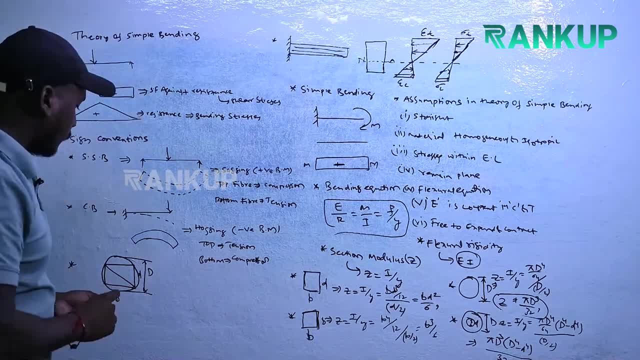 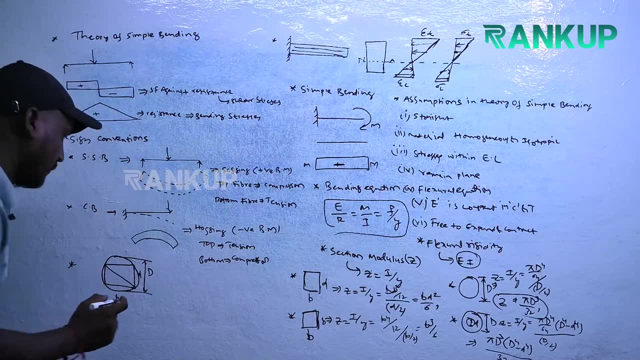 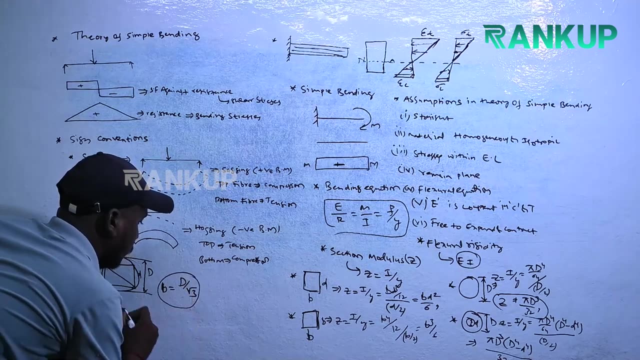 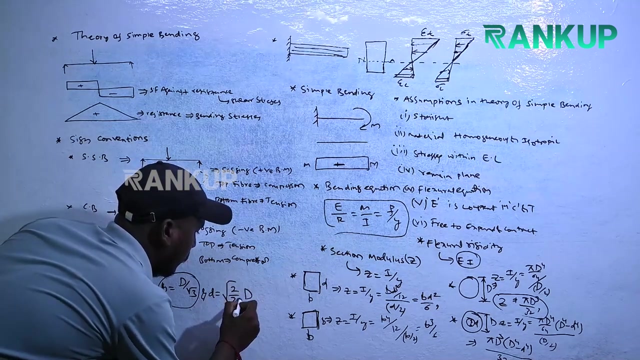 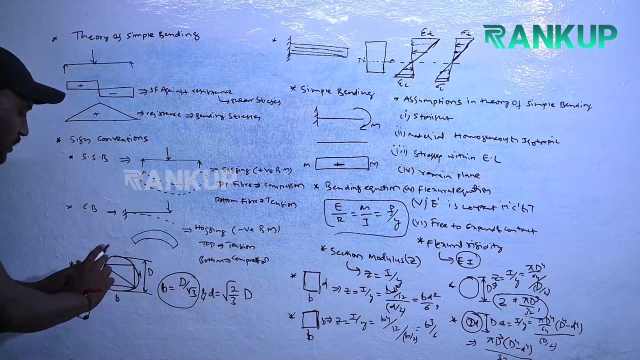 Okay, strongest beam cut out of the circular section. the dimensions small b is equal to capital d divided by square root 3, and depth of the beam is square root of 2 by 3 into capital d. the dimensions for the strongest beam which is cut out of a circular section is b is equal to d by square root 3, capital d by.